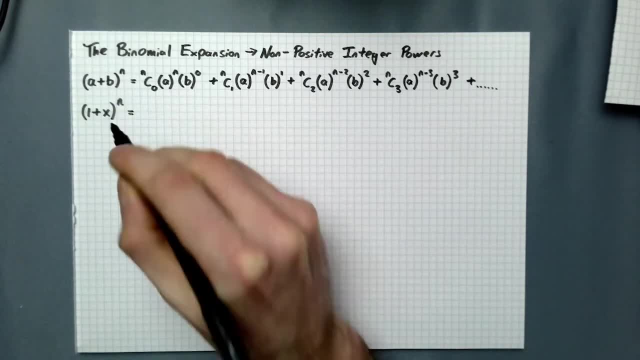 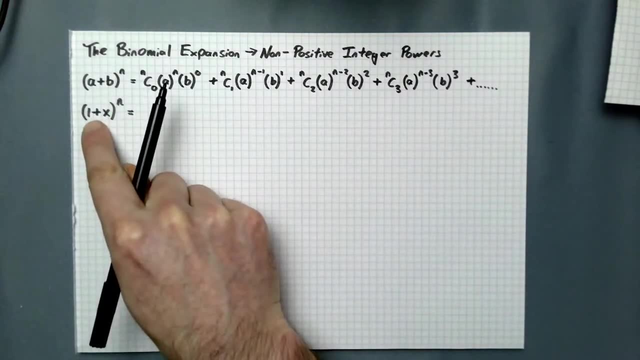 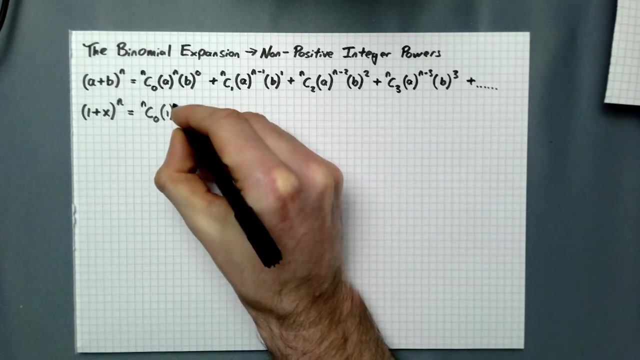 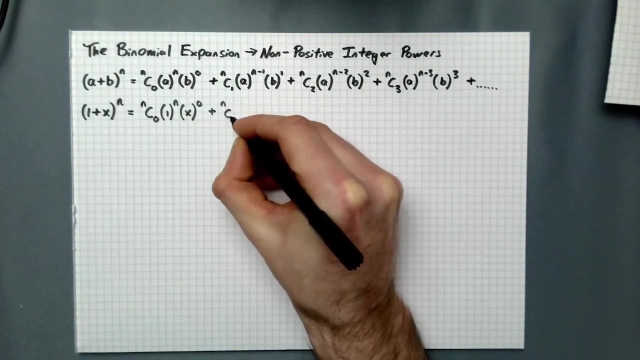 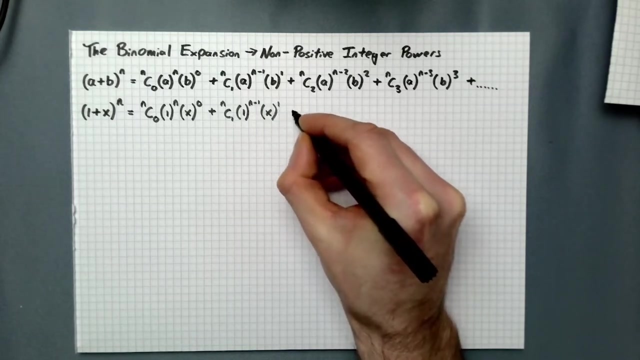 one plus x, same thing to the power of n. and I insert everything into this formula here. Let's see what happens. So, inserting in my one for a and my x for b, I get n- c naught. one to the n, x to the zero plus n, c, 1, one to the power of n minus one times x to the power of one. 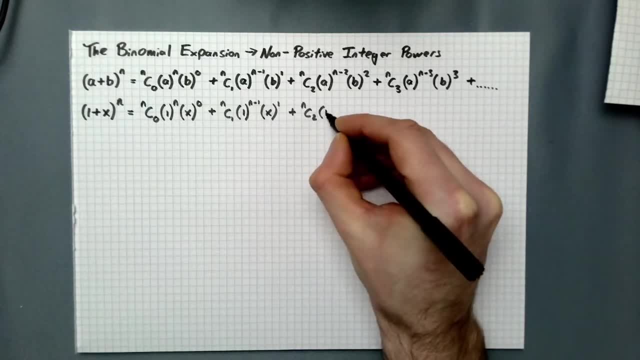 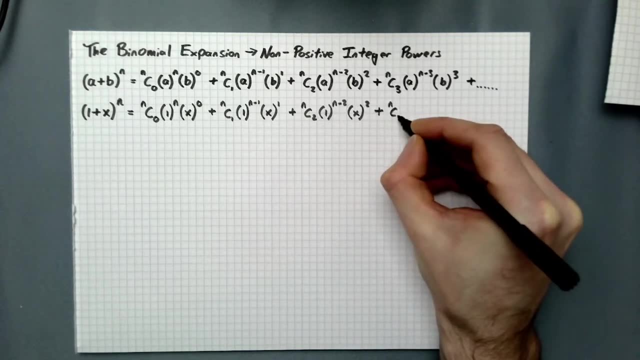 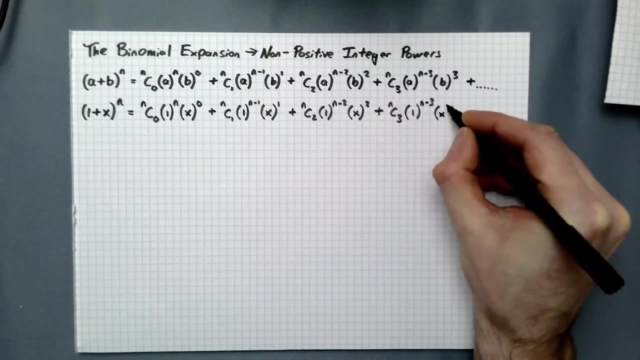 plus n c 2, one to the power of n minus zero, plus n c 1, plus n c 2, one to the power of n minus one of n minus 2 times x squared, plus nc3 times 1 to the power of n minus 3 times x cubed, and this: 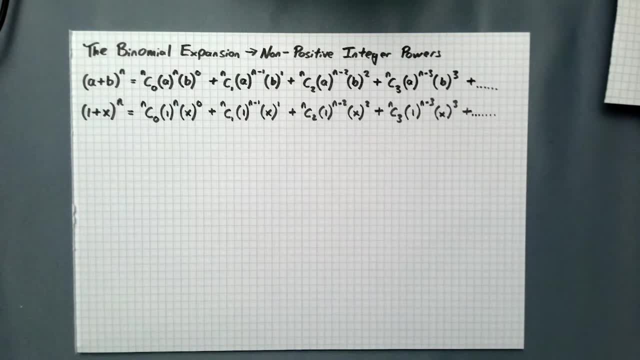 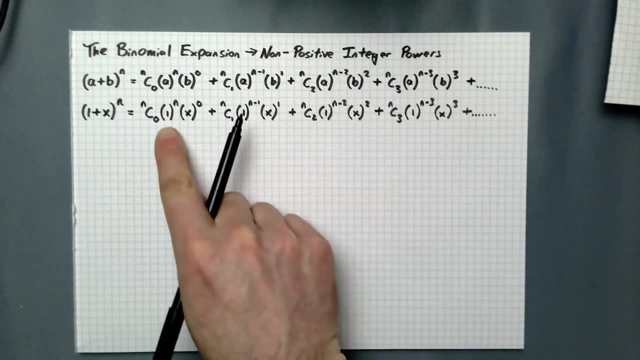 this pattern will kind of continue on and on and on. Okay, so I'll get to work tidying this up now. I know that 1 to the power of anything is just going to be 1, so all of these 1 terms will have. 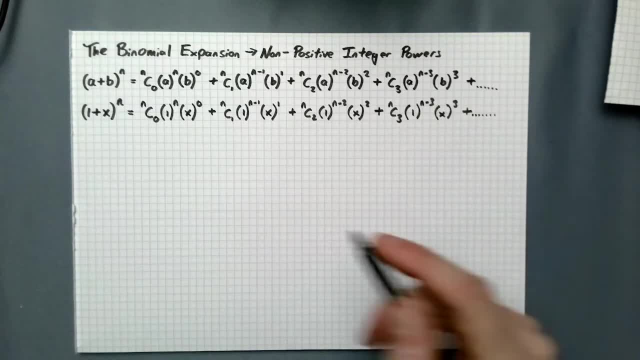 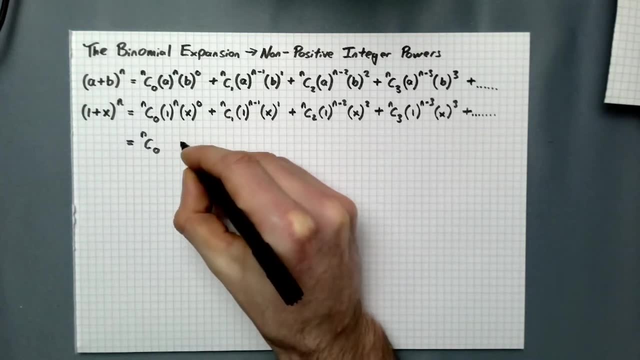 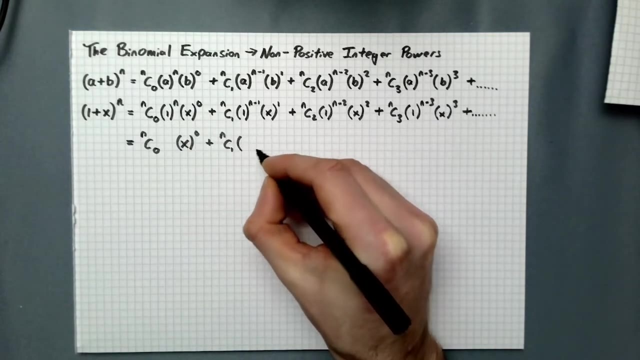 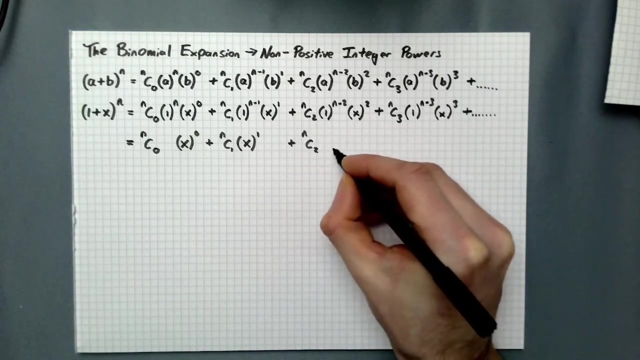 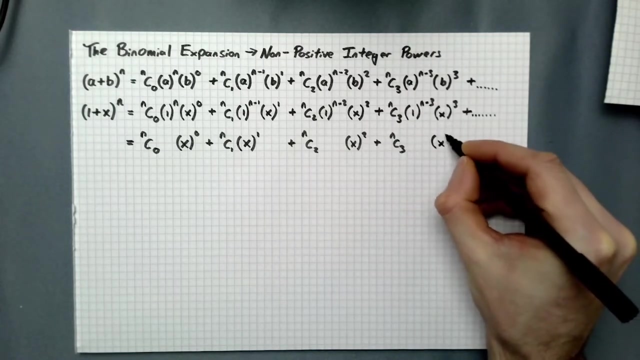 no real, no real effect here. I can essentially just eliminate them. So I'm going to rewrite this as: nc naught times x to the naught, plus nc1 times plus x to the 1, plus nc2 times x squared, plus nc3 times x cubed, plus carrying on and on and on. Okay, so to continue tidying this up, I now want to. 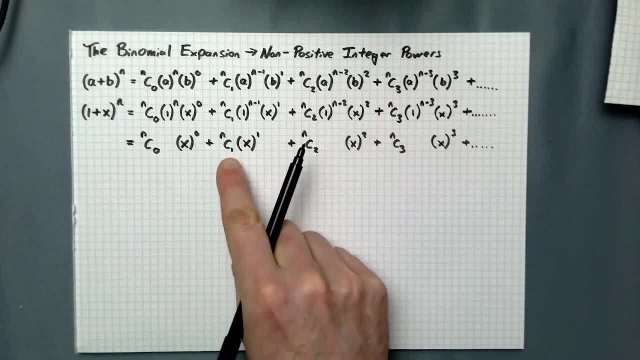 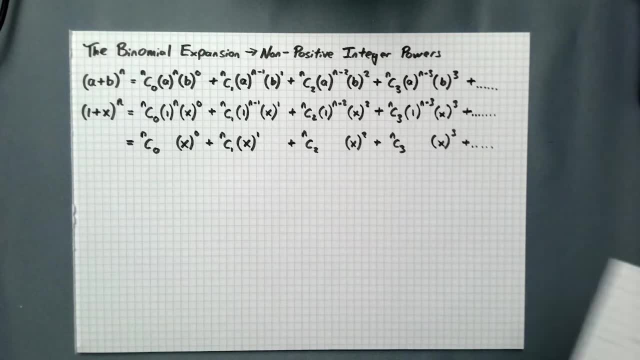 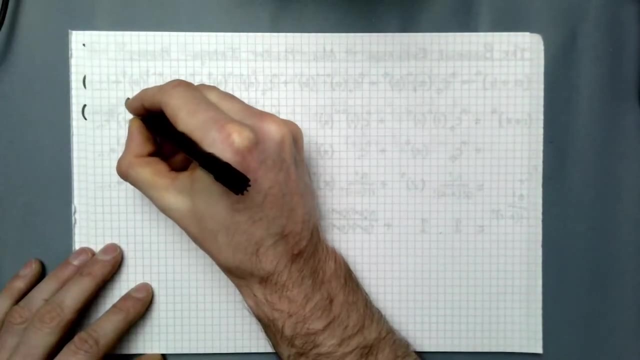 kind of come out of some generalized expression for these nc naughts, these nc1s, nc2, nc3, and I'm going to kind of give a demonstration on a separate bit of paper here. So suppose I want to work out, let's say, 6c3. 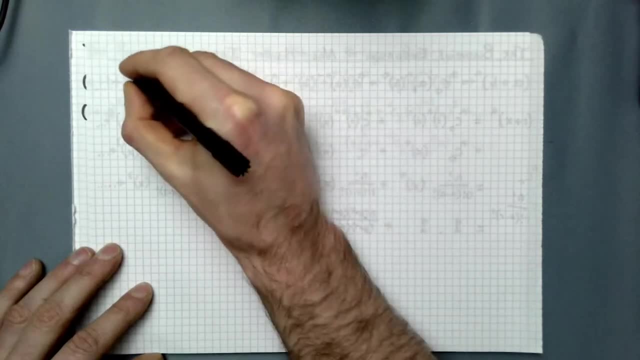 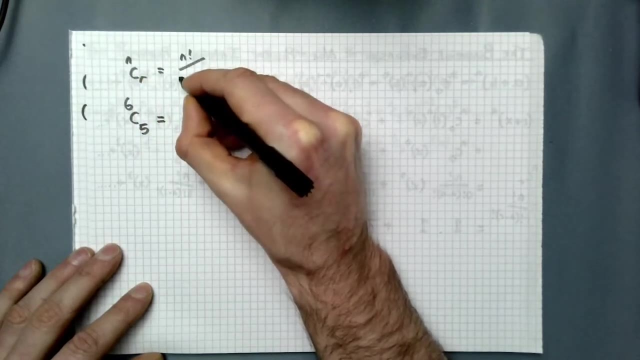 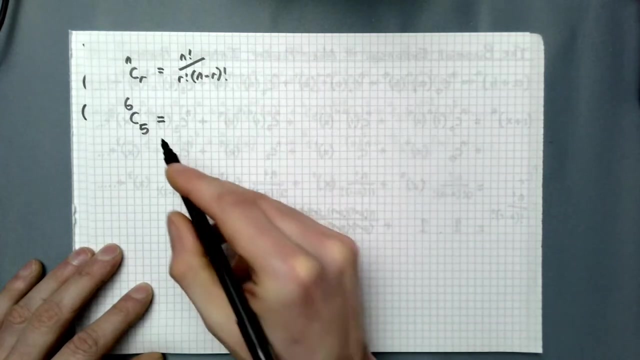 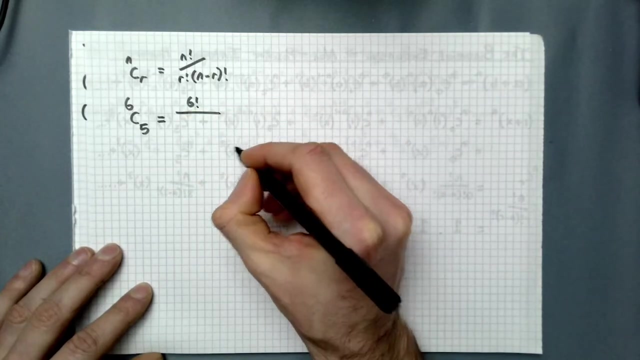 5.. Well, I know that my general formula for combinations ncr is n factorial over r factorial, times n minus r factorial. So if I wanted to work out 6c5, I could say 6 factorial over 5 factorial, 6 minus 5. 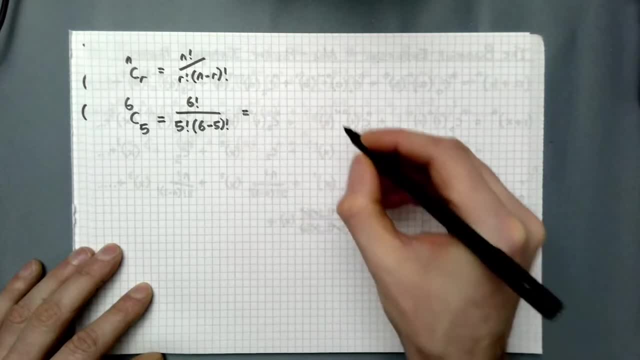 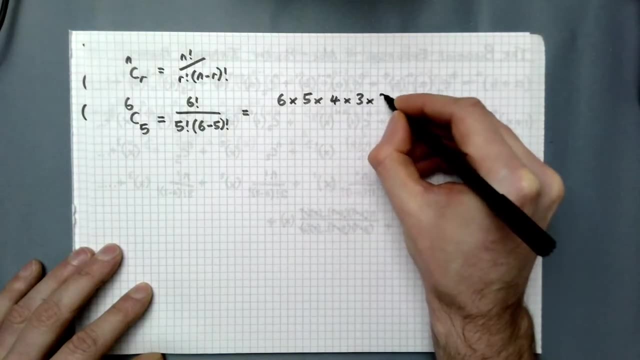 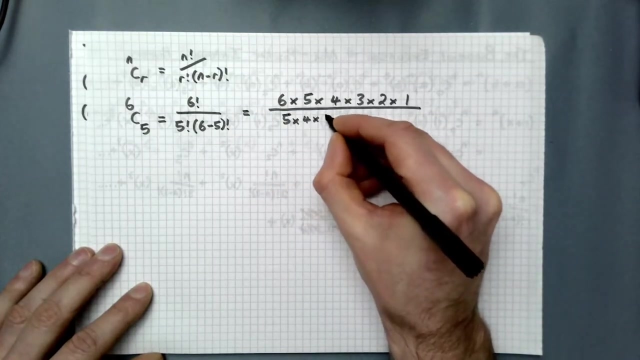 factorial, which tidies up nicely. 6 factorial is 6 times 5 times 4 times 3 times 2 times 1, all over 5 factorial, which is 5 times 4 times 3 times 2 times 1 times 6 minus 5 factorial, or 1 factorial. 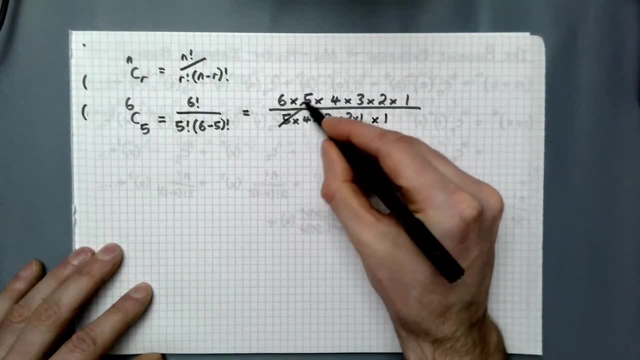 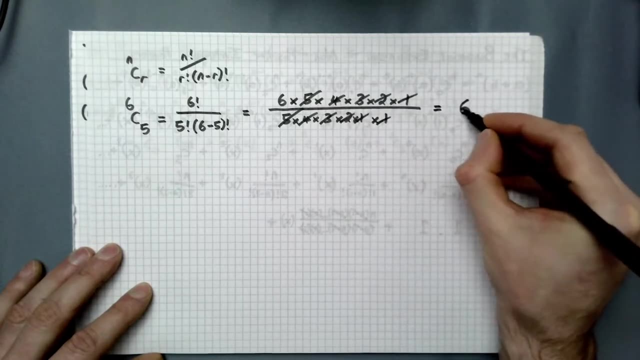 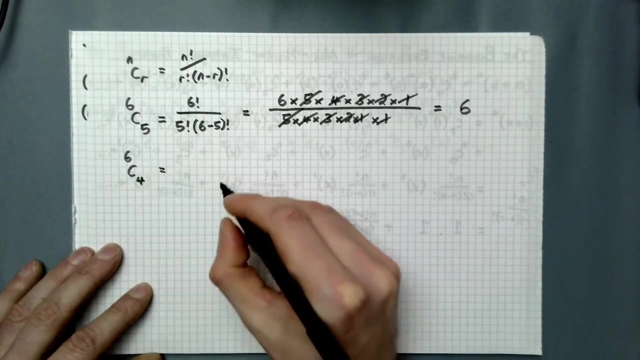 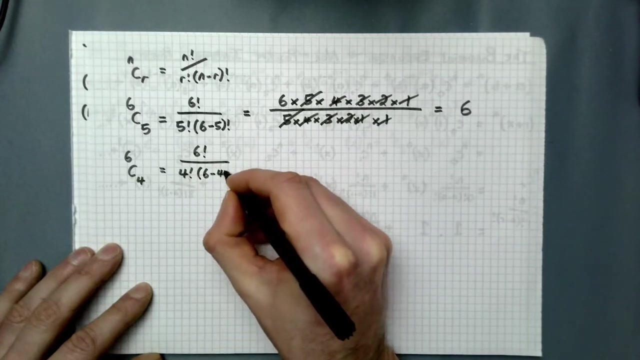 that's just another 1.. So what happens? pretty much all of these terms factorial is always going to cancel down very nicely and I'm left with my answer, which is just 6.. Suppose I wanted to do this with 6c4, so that would be 6 factorial over 4 factorial, 6 minus 4 factorial. So this is. 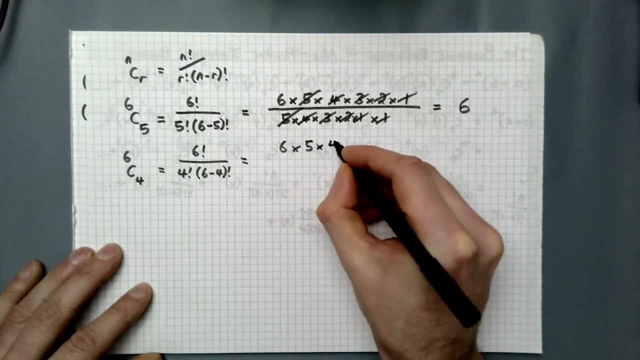 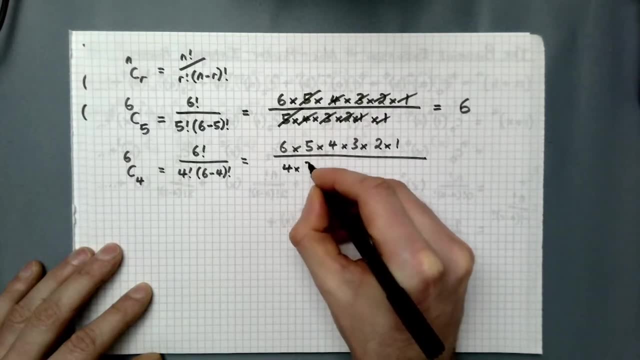 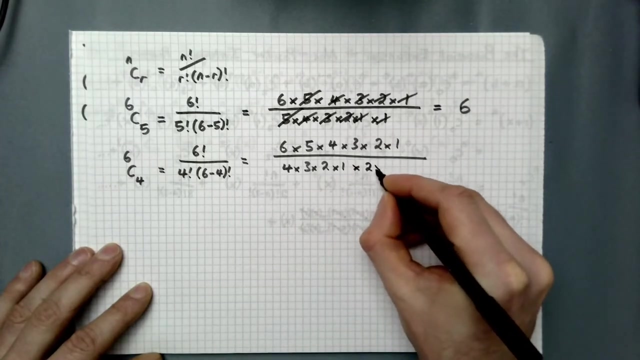 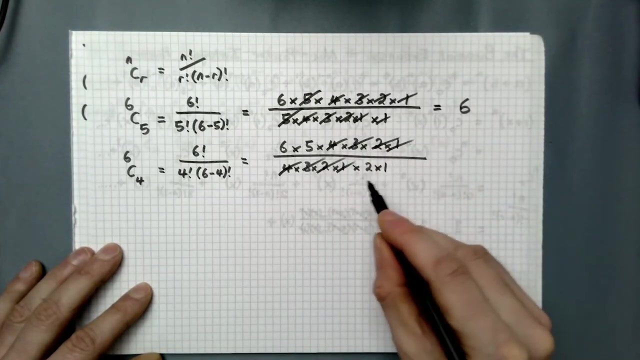 going to give me 6 times 5 times 4 times 3 times 2 times 1.. Elliott has done the following. My answer would be that now, of course, will be 2 times 5 times 2 times 1, all over 4 factorial, which is 4 times three times 2 times 1 times 6 minus 4 is 2.. 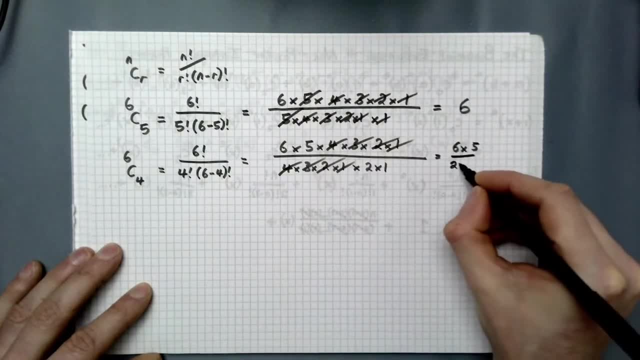 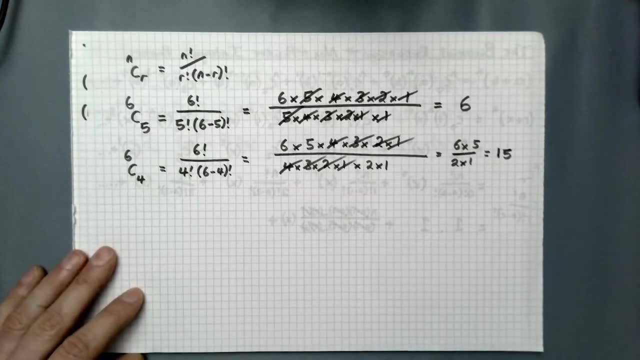 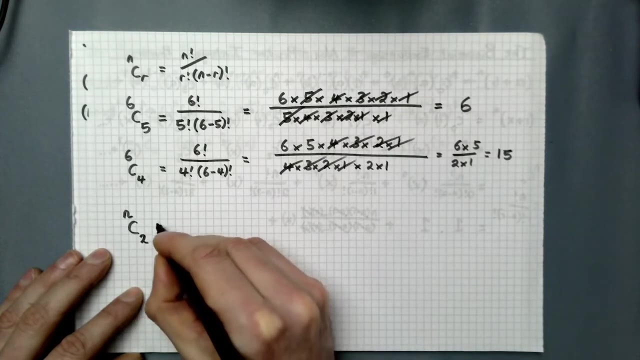 2 factorial is 2 times 1. so cancel, cancel, cancel. And then I'm left with 6 times 5 over, 2 times 1 DM gossiping against the evidence. register algebra as well, Suppose I want to work out nc2.. So this is going to be n factorial over. 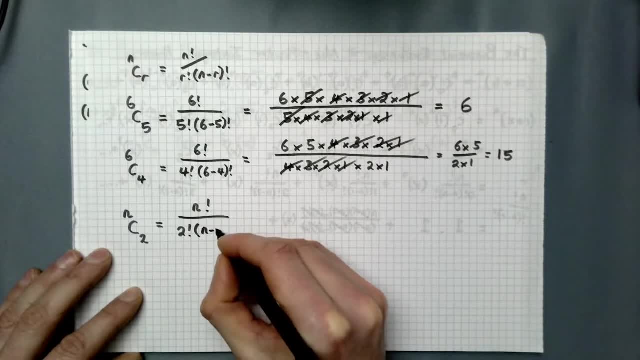 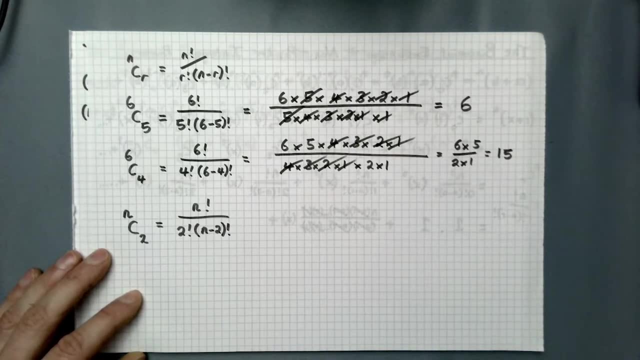 two factorial, n minus two factorial, And it might look as if this won't simplify because the n becomes quite problematic. but factorials always have this kind of fantastic pattern that a factorial just means you take a number and you multiply that number by every integer. 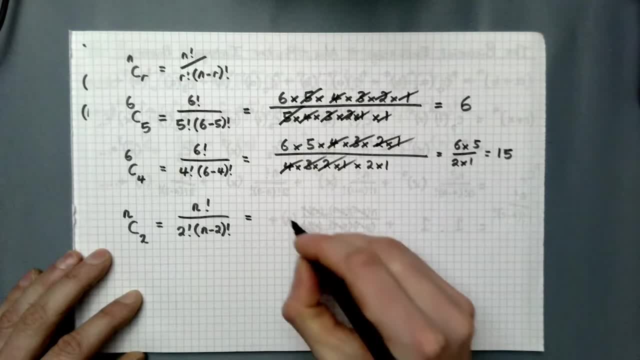 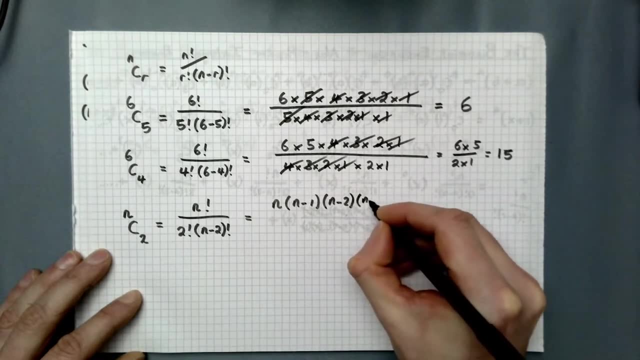 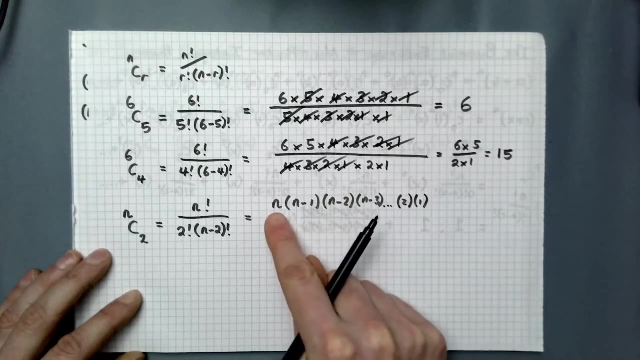 beneath it all the way down to one. So n factorial is just going to be n times n minus one, times n minus two times n minus three, all the way down to one. So I've kind of skipped out a few steps here. It doesn't matter what n is, I know it's going to carry on all the way. 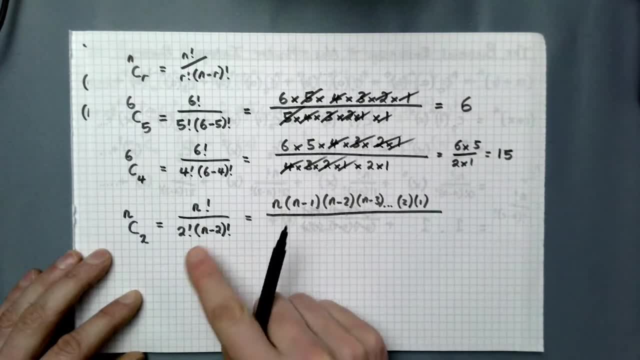 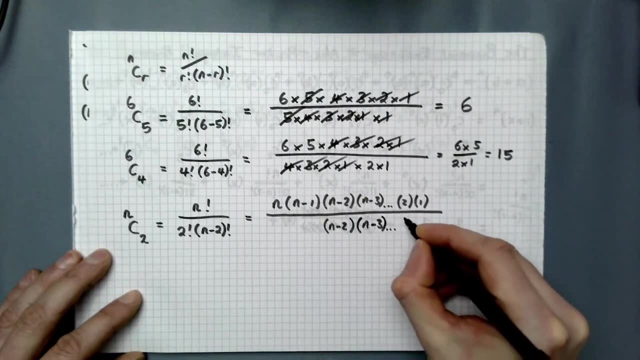 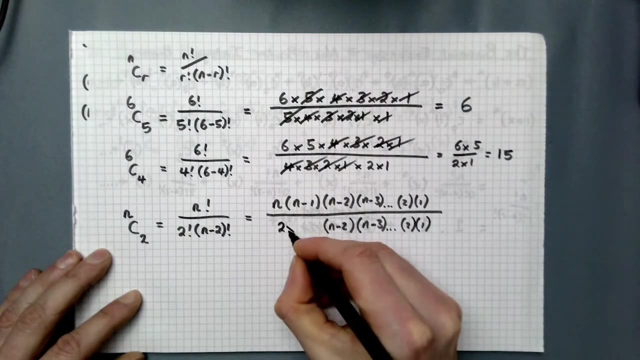 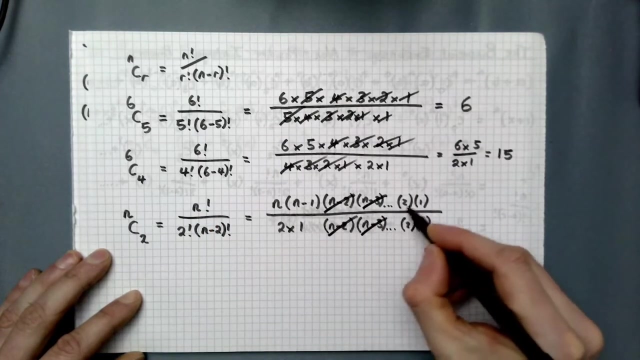 down to one …. n minus 2. factorial is just going to be n minus 2 times n minus 3, all the way down to 2 times 1.. And 2 factorial is just 2 times 1.. So the great thing about factorials: even if they're in terms of n, they still simplify massively. 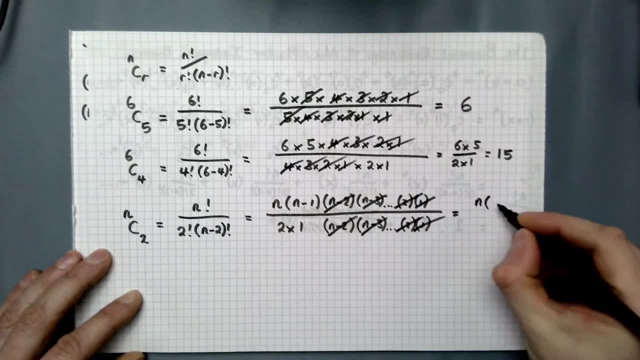 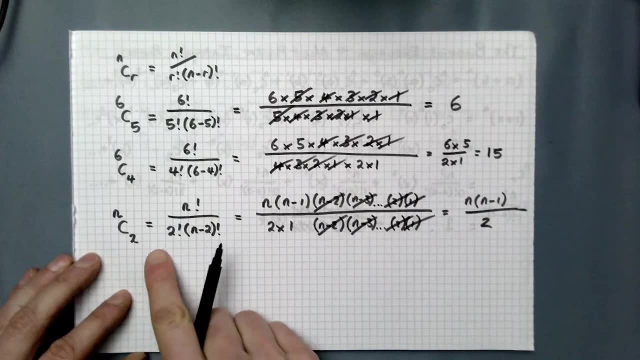 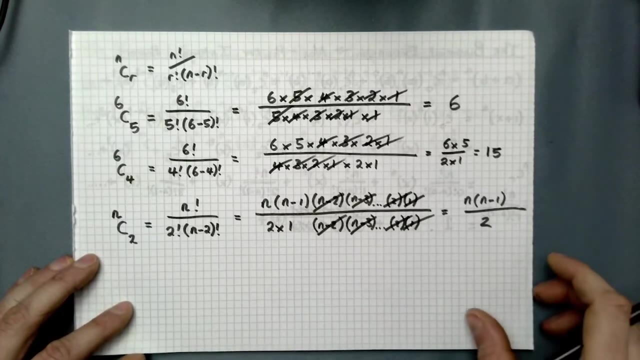 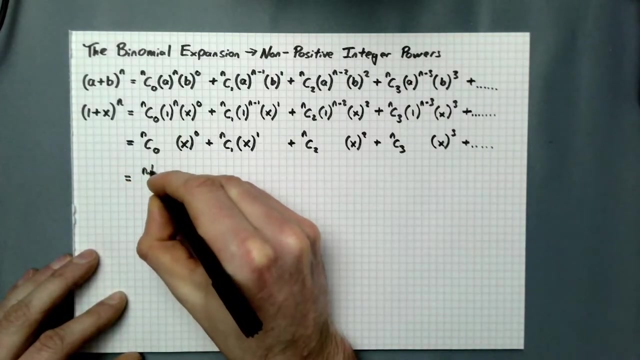 So I'm left with n times n minus 1 over 2 for nc2. here Now I'm going to apply this logic to all of my terms within this binomial expression, binomial expansion expression, which I'm looking to simplify, So I can say that nc0 is n factorial over 0, factorial n minus 0.. 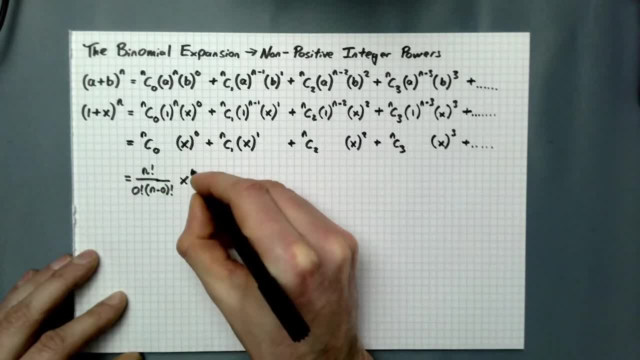 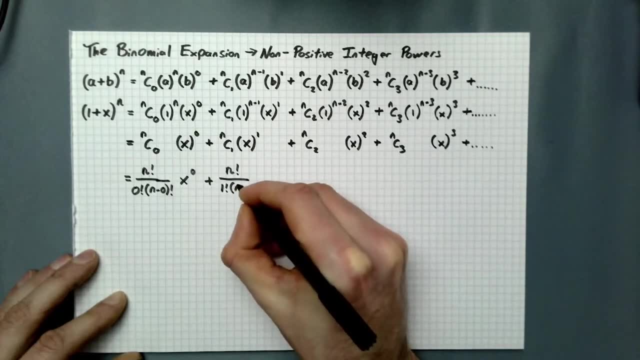 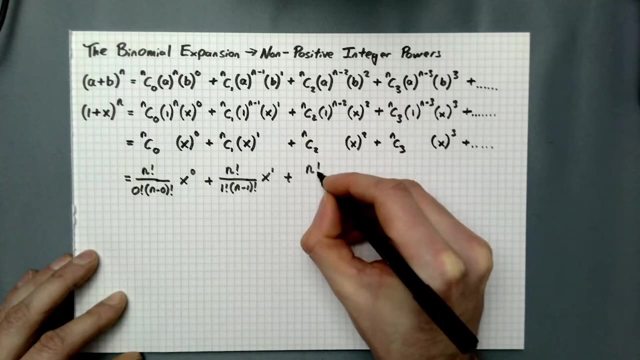 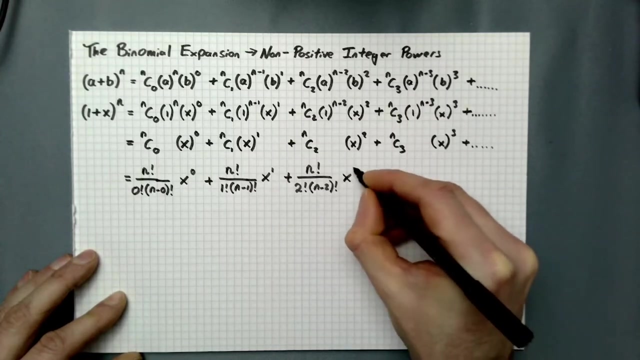 Factorial, and this is all times by x to the 0.. Plus nc1,, which is n factorial over 1 factorial. n minus 1 factorial times x to the 1.. Plus nc2,, which is n factorial over 2 factorial. n minus 2 factorial, all times by x squared. 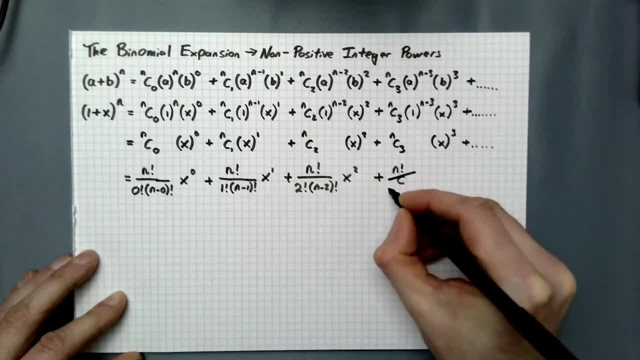 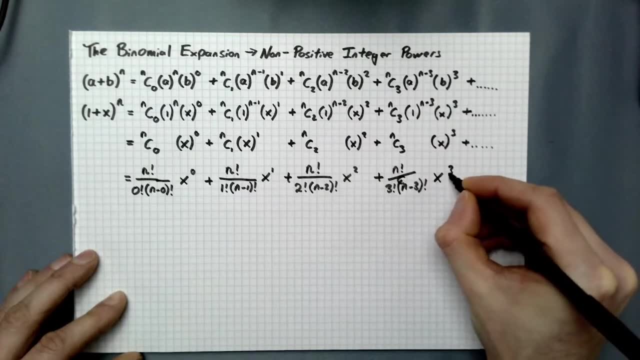 Plus nc3, which is n factorial Plus n factorial over 3 factorial. my apologies, handwriting error: n minus 3 factorial times by x cubed, And this pattern will continue on. So n factorial, 0 factorial is 1.. 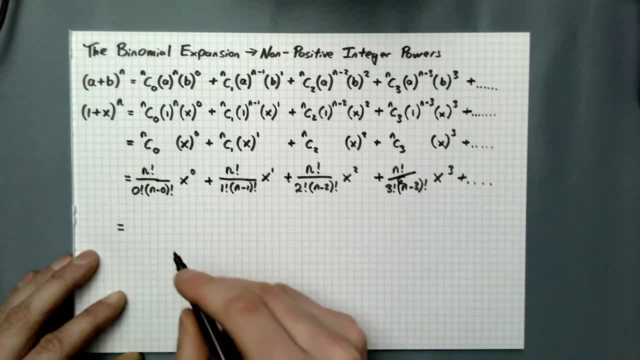 n factorial over n minus 0, which is just n factorial. again, This is just 1 times by x to the 0, anything to the power of 0 is 1.. So this first term here is 1.. Plus n factorial over n minus 1 factorial. 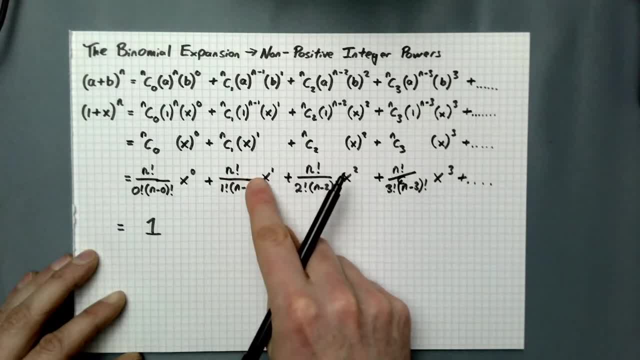 Plus n factorial over n minus 1 factorial. So I know that this is n times n minus 1 times n minus 2 times n minus 3.. This is n minus 1 times n minus 2 times n minus 3.. So everything is going to cancel except n and this 1.. 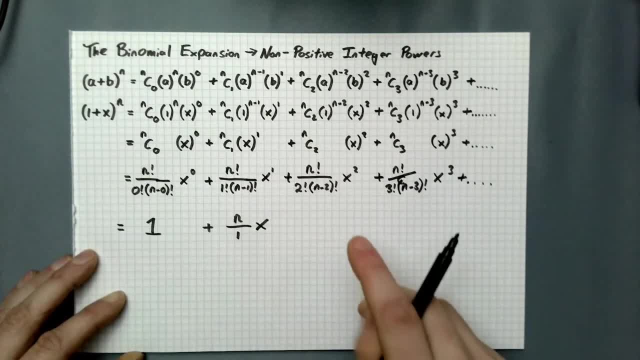 And this is all being multiplied by x. Here I've got n times n minus 1, times n minus 2, times n minus 3.. This is n minus 2 times n minus 3, times n minus 4, all the way down to 1.. 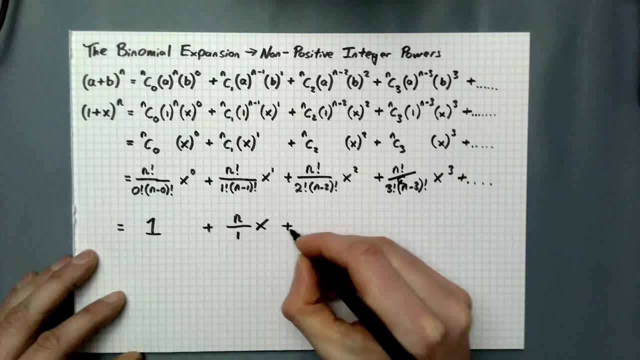 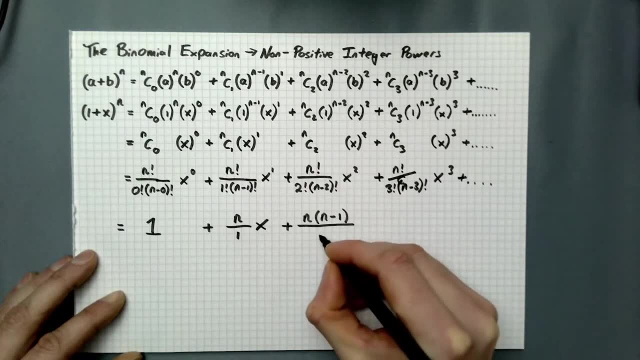 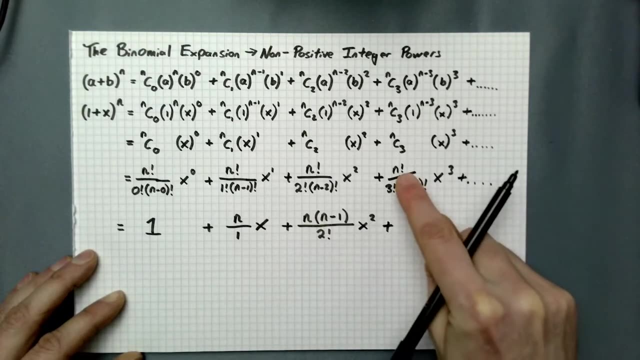 So I'm going to do this, I'm going to have a lot of cancellations And I'm going to be left with n times n minus 1 all over 2 factorial. And this is times by x squared Plus n factorial over n minus 3 factorial. 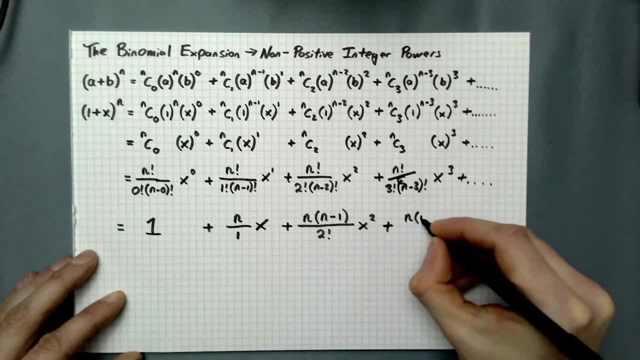 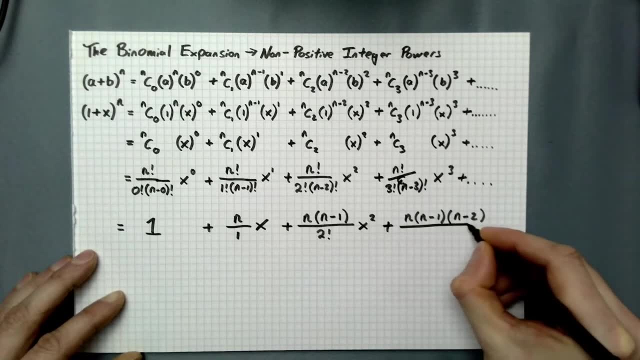 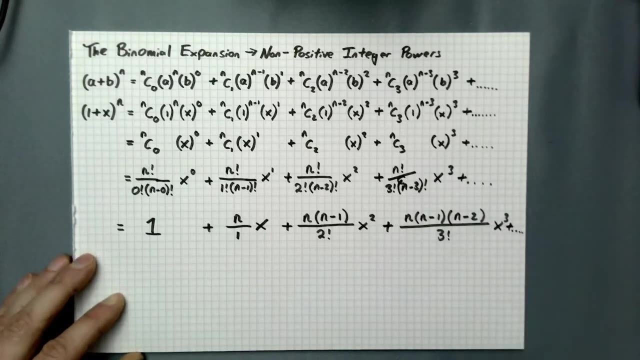 So everything is going to cancel except the n, the n minus 1, and the n minus 2.. And on the denominator, I'm just going to be left with the 3 factorial. And this is all times by x cubed. 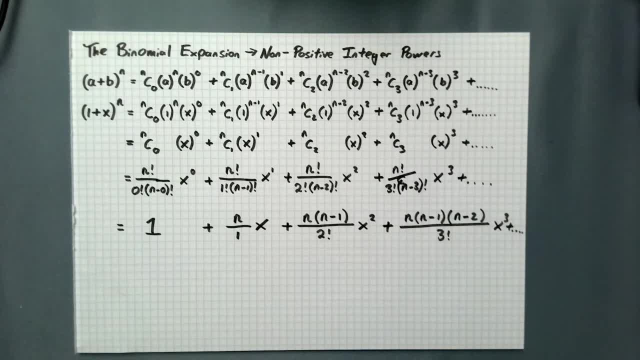 And this pattern continues on and on. So we have an alternative formula for the binomial expansion here, But this formula will only work if we have a 1 as our leading term within our expansion to make here. So in the next part of this video I'm going to do some demonstrations of this. 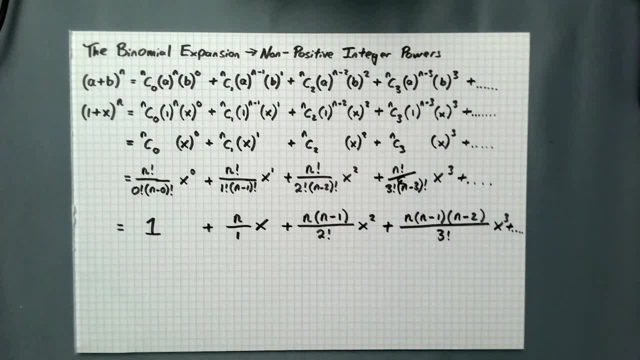 I'm going to see what happens Using some nice integer positive integer powers using our original formula and this new formula, And then I'm going to test out this new formula using a non-positive integer power. In a later video I'll do loads of examples, so feel free to follow along for part 2.. 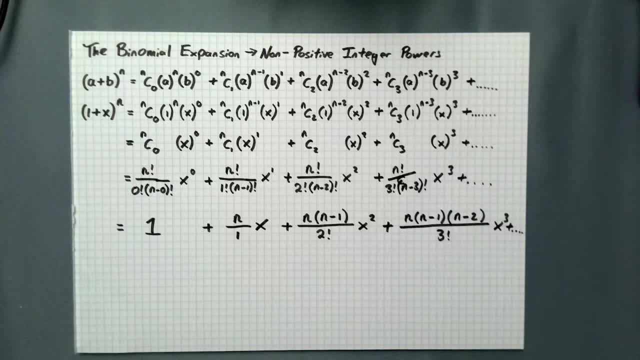 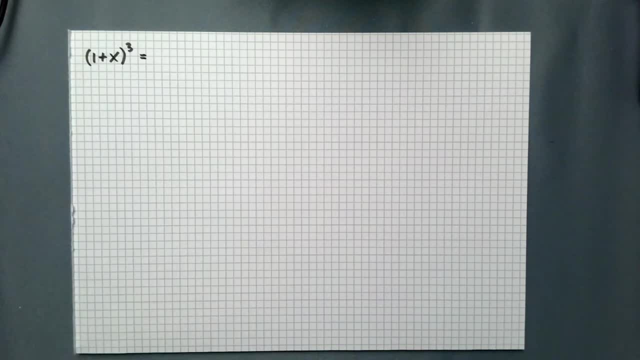 And we'll get up to speed with this topic. I'll see you then. Okay, part 2.. I'm going to work through this fairly simple example: 1 plus x, all cubed using the old formula, And then I'm going to test out the new formula which I developed in part a. 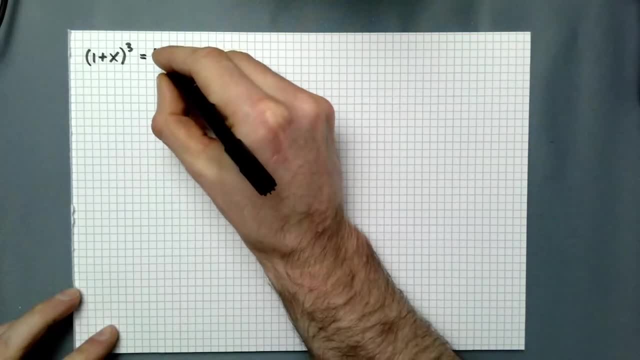 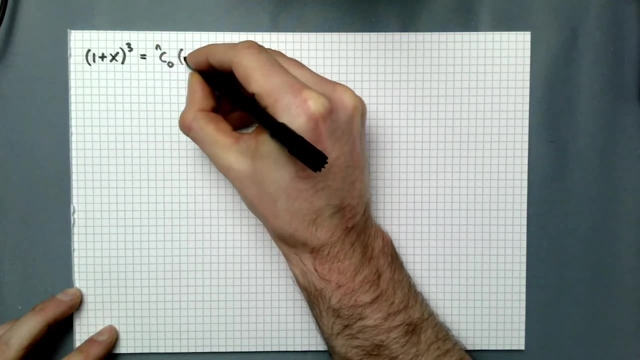 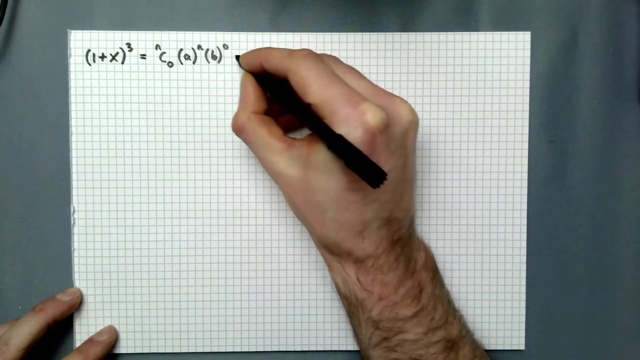 So for this formula here I'm going to say nc0 times by my old formula. I'll write out the old formula, So nc0 times a to the n, times b to the 0.. Plus nc1 times a to the n, times b to the 0.. 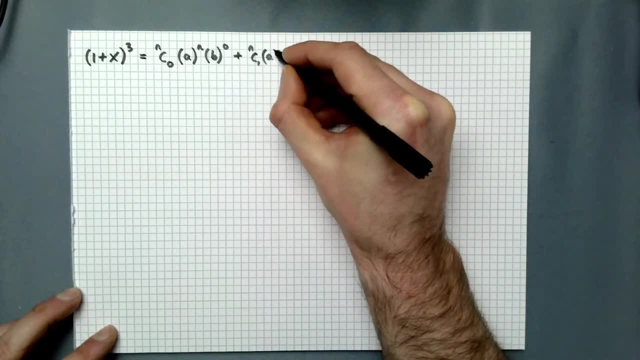 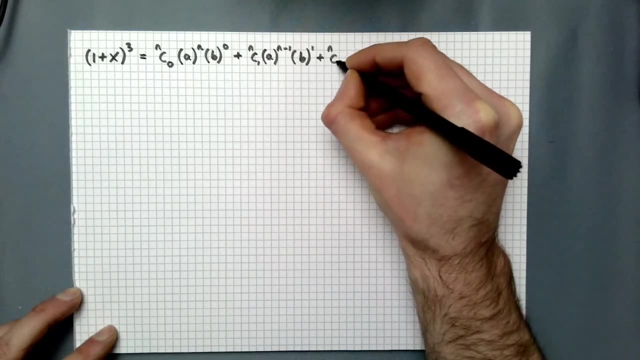 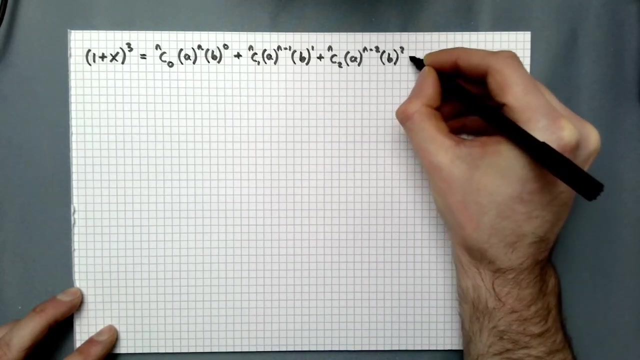 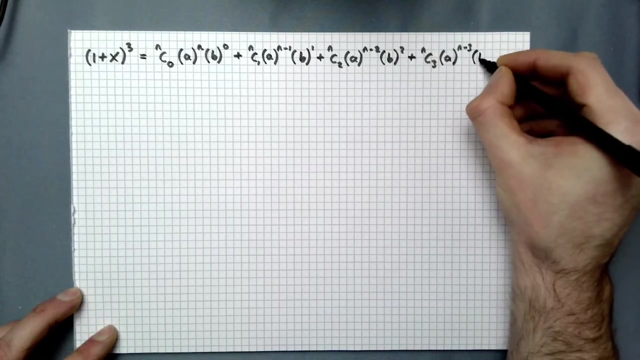 Plus nc1 times a to the n times b to the 0.. Plus nc2 times a to the n minus 1 times b to the 1.. Plus nc2 times a to the n minus 2 times b squared. Plus nc3 times a to the n minus 3 times b cubed. 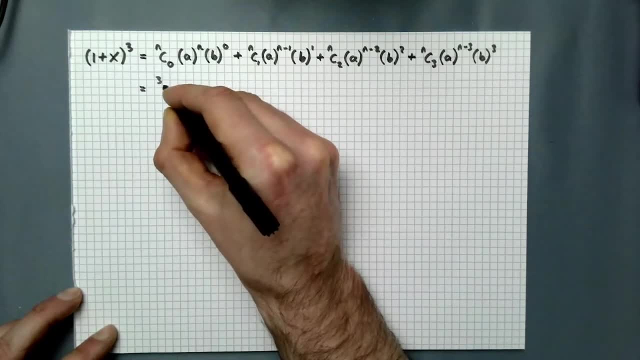 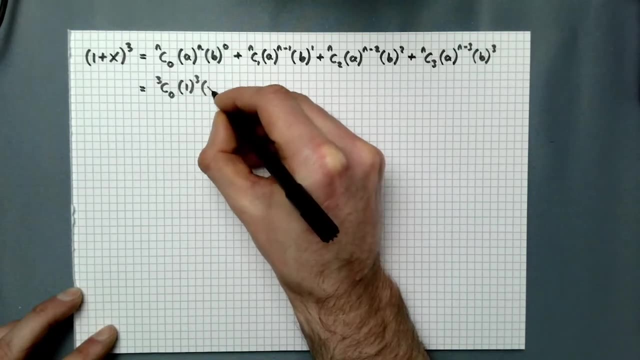 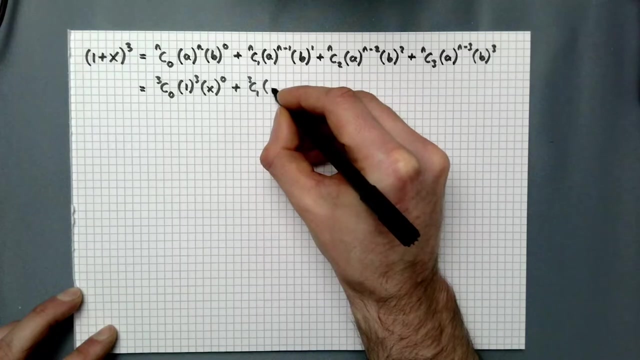 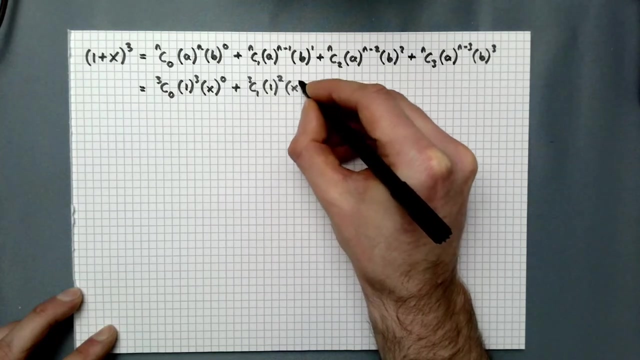 So I'll insert all my terms in. So 3c0 times by a, which is 1 to the power of 3 times b, which is x to the power of 0. Plus 3c1, which is sorry, times 1 to the power of 3 minus 1, which is 2 times b, which is x to the power of 1.. 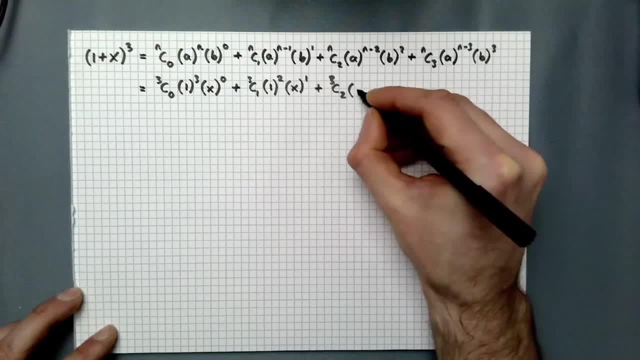 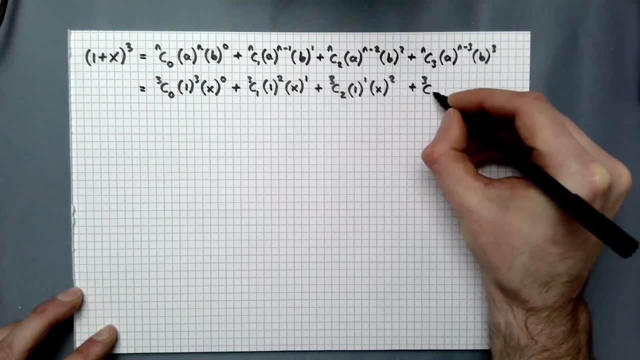 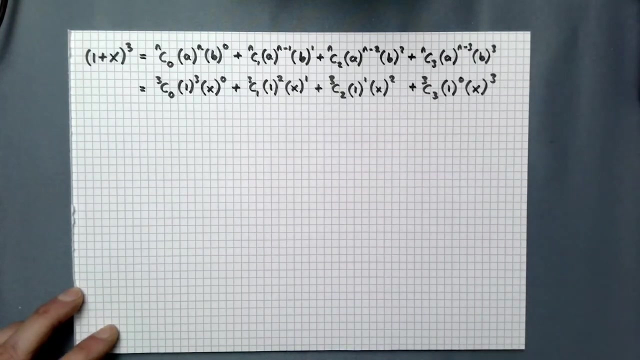 Plus 3c2. times by 1 to the power of 1.. Times by x all squared, Plus 3c3,, 1 to the power of 0, x all cubed, So 3c0,. so I can do these using Pascal's triangle if I wanted. 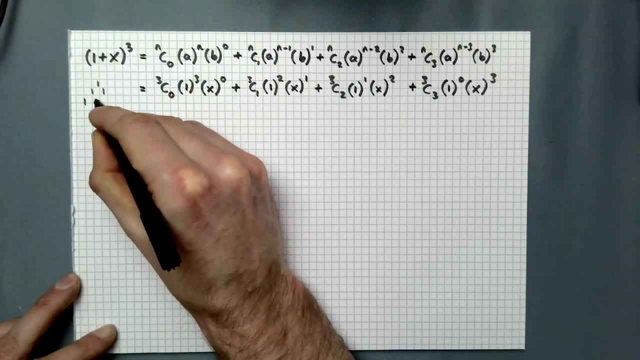 So Pascal's triangle, little one down the side here- So 1, 1, 1, 1, 2, 1, 1, 3,, 3, 1.. So this is 1.. 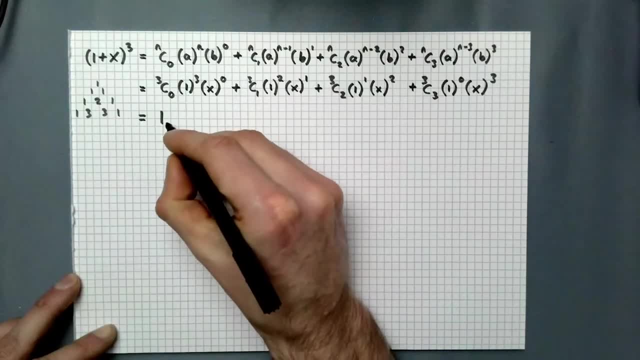 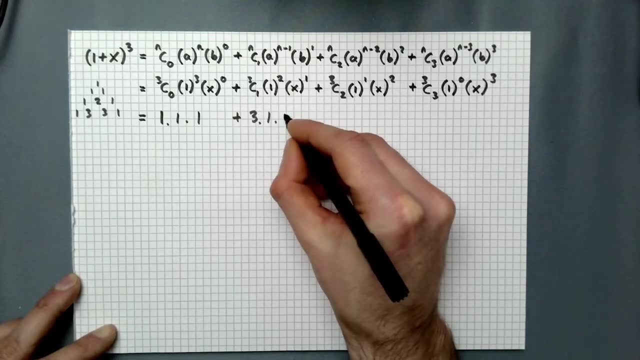 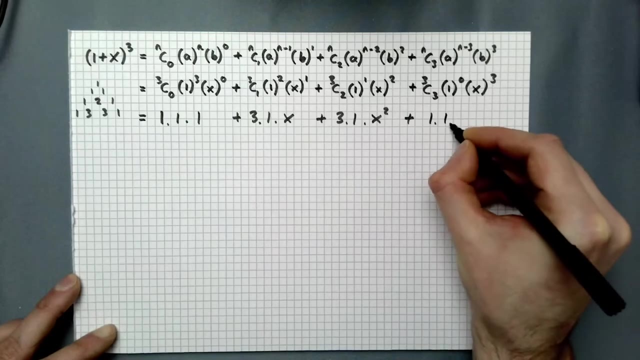 So here's my coefficients, just here. So 1 times 1 cubed times x to the 0, which is 1.. Plus 3 times 1 times x, Plus 3 times 1 times x squared, Plus 1 times 1 times x cubed. 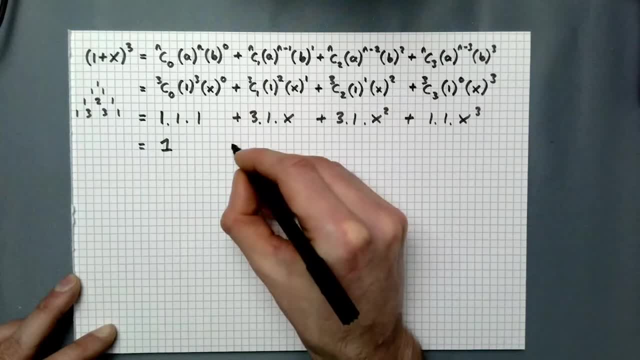 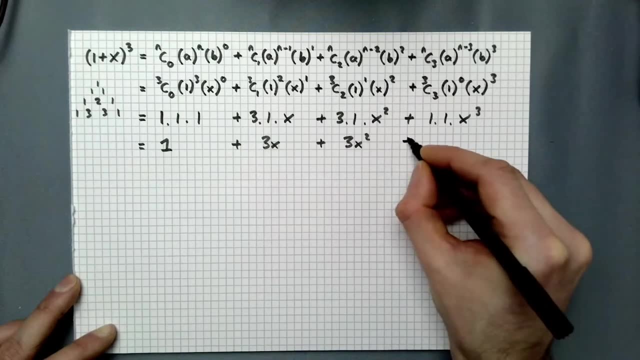 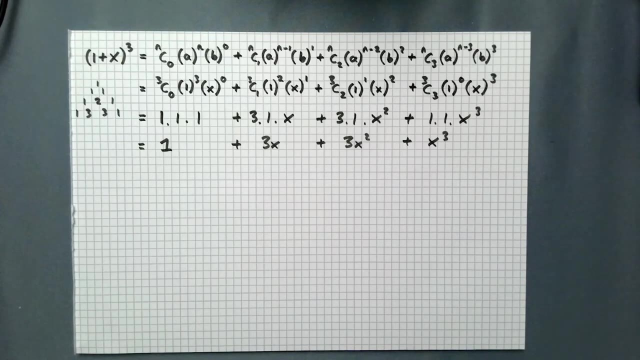 Which gives me my final answer of 1 plus 3x plus 3x squared plus x cubed. So let's test this out using our alternative formula, the one we developed in part A. So I'll put a little line under here, just so we can separate everything out. 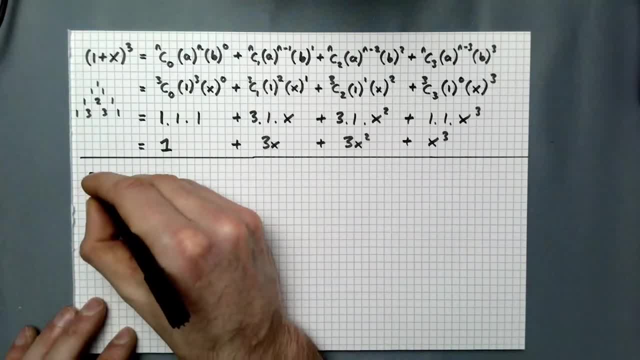 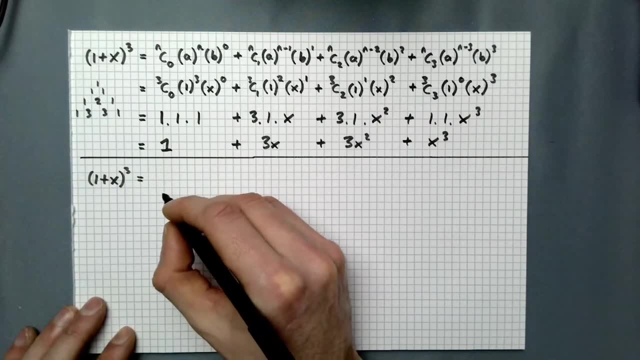 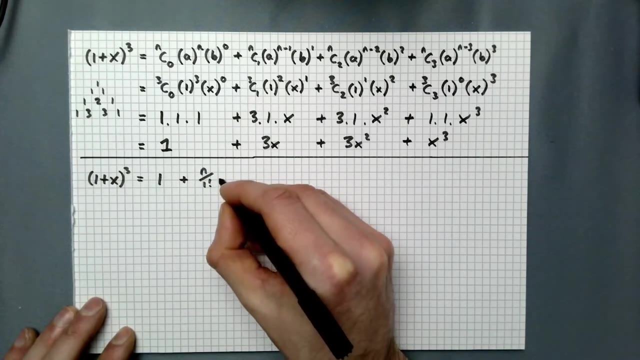 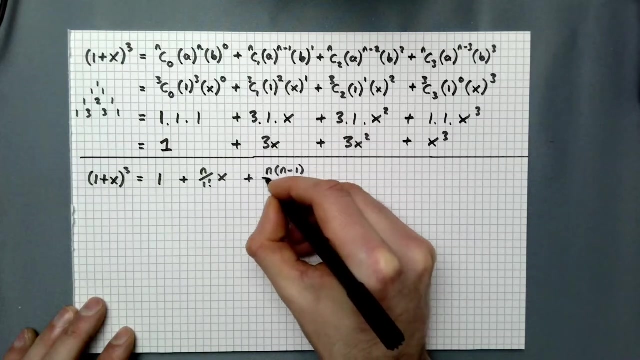 So I'm going to test out my new formula here. So 1 plus x, all cubed is equal to. I'll write out the formula: So 1 plus n over 1 factorial times by x Plus n times n minus 1 over 2 factorial times x squared. 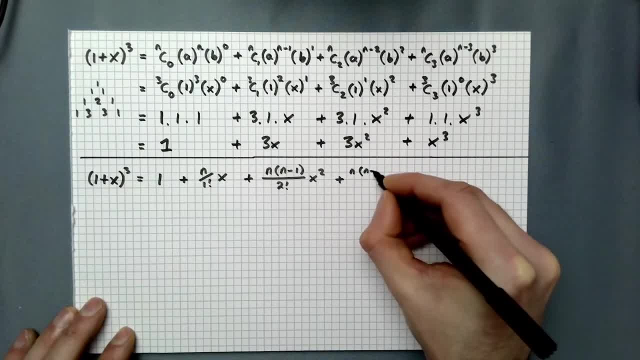 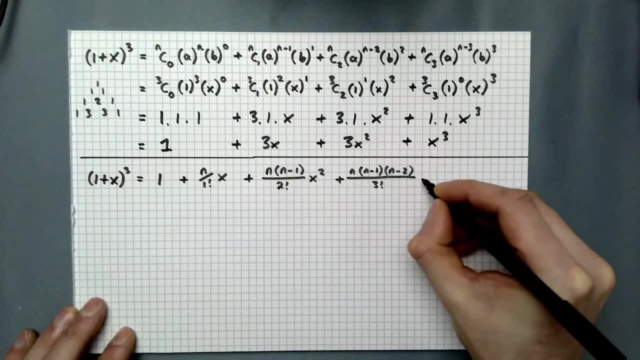 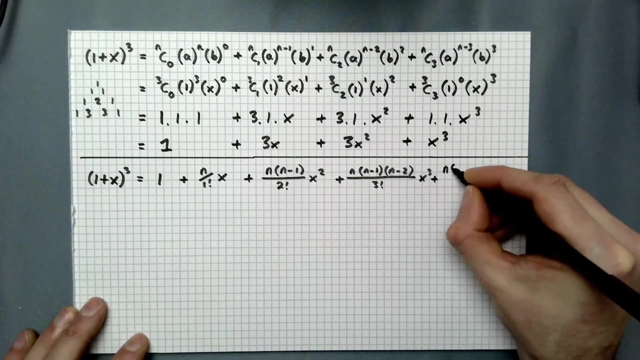 Plus n times n minus 1 times n minus 2 over 3 factorial x, cubed Plus, and this carries on and on and on, forever, remember. So I'll have to keep going and going. So n times n minus 1 times n minus 2 times n minus 3, all over 4 factorial x to the 4.. 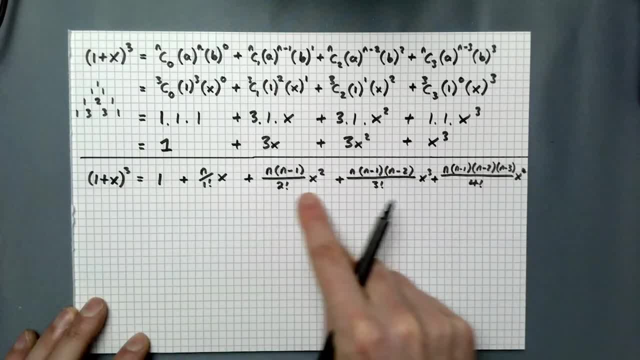 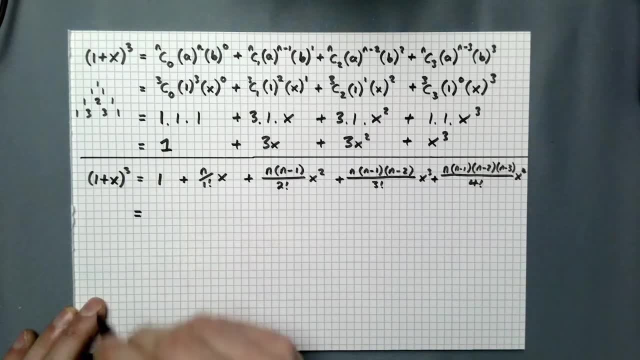 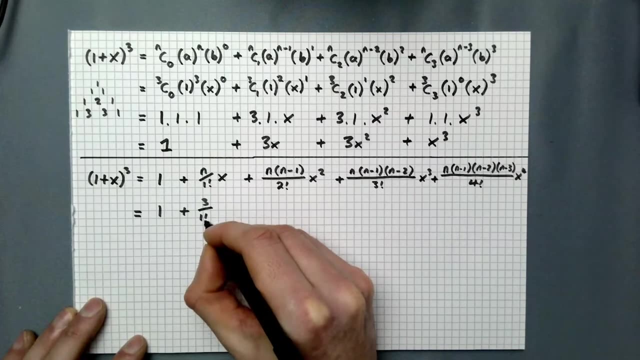 I obviously have to kind of carry on forever with this formula, But I'm kind of running out of space so I'll go up to this term here. Something interesting will happen by this point, I promise. So 1 plus 3 over 1. factorial times x. 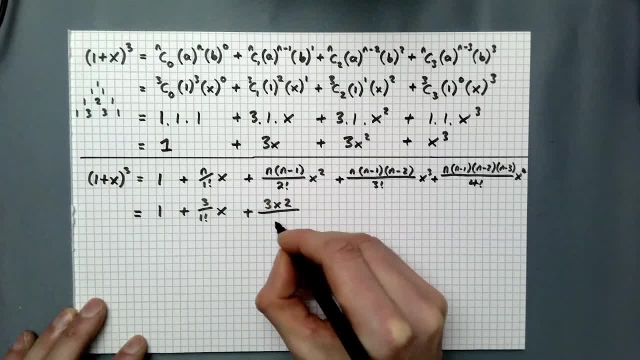 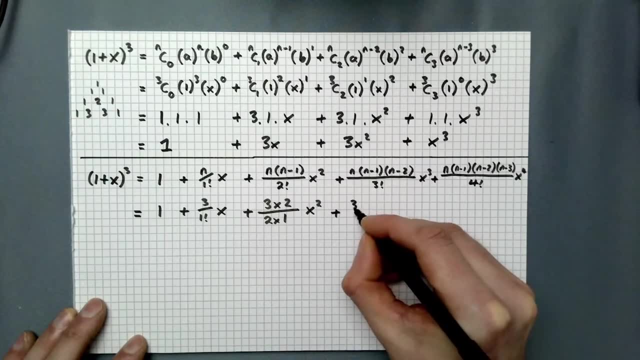 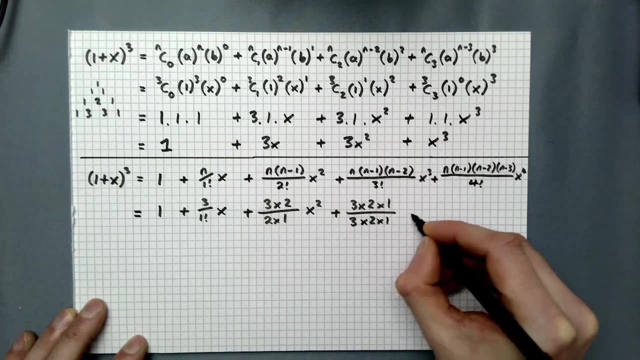 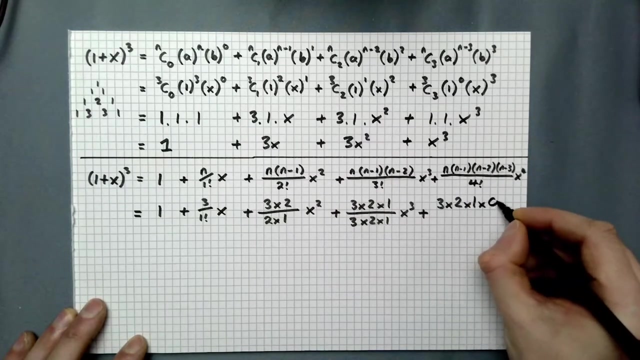 Plus 3 times 2 over 2 times 1 x squared Plus 3 times 2 times 1 over 3 factorial, which is 3 times 2 times 1 x cubed, Plus 3 times 2 times 1 times 0 over 1 times 2 times 3 times 4.. 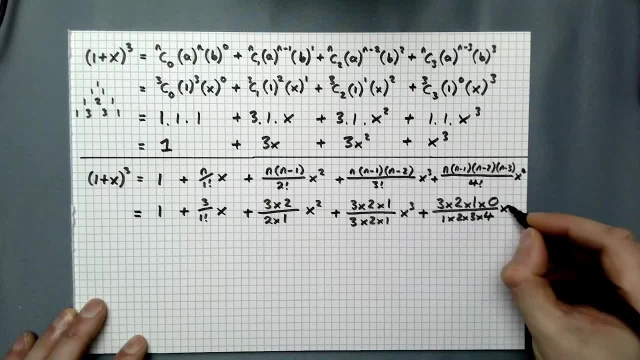 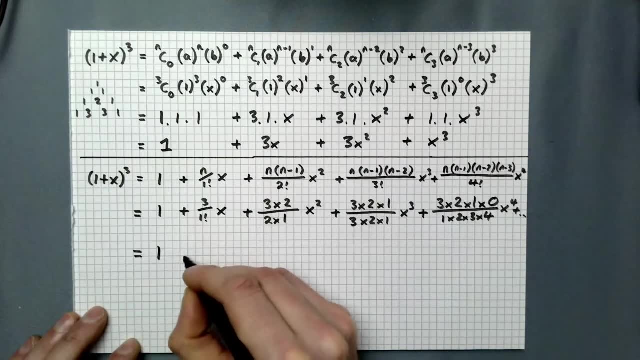 I realise I've just wrote it the wrong way round, but it makes no difference. Times x to the 4 plus carrying on, and on, and on. So I can tidy up each of these terms. So 1 plus 3 over 1 factorial gives me 3 x. 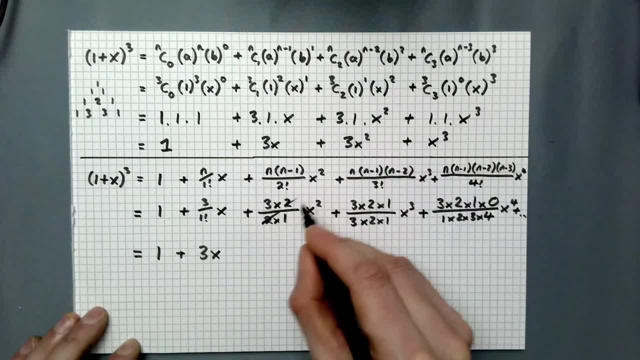 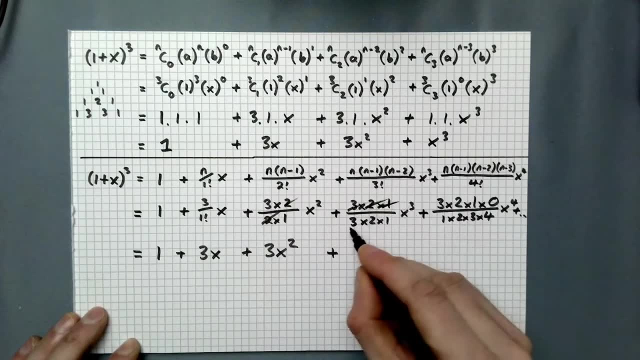 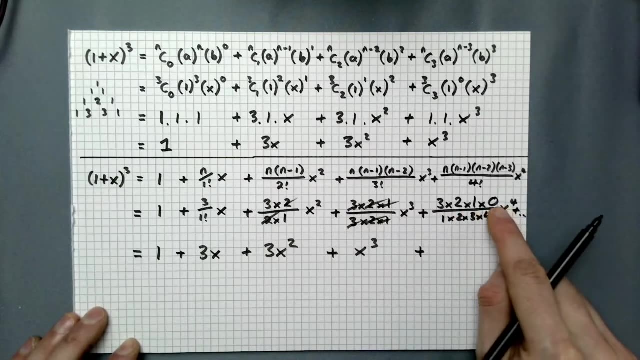 3 times 2 over 2 times 1, 2's cancel gives me 3 x squared Plus 3, 2, 1, 3, 2, 1 leaves me with x cubed And over here I've got 3 times 2 times 1 times 0.. 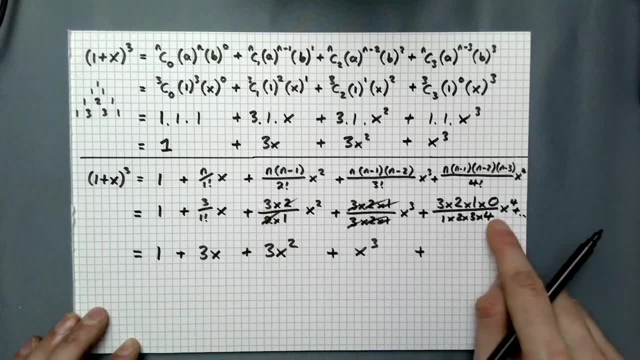 So this whole expression here, this whole term here, is going to be 0.. So 0 x to the 4.. And because when I carry on this pattern, if I were to keep saying n times n minus 1 times n minus 2, times n minus 3 times n minus 4 times n minus 5.. 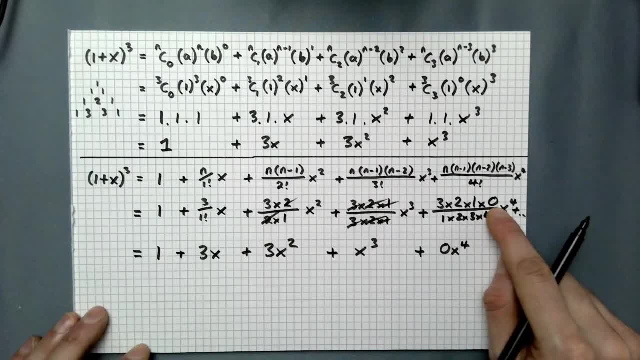 I will always have a 0 term in my numerator, So any coefficients beyond this point are going to be 0 as well. So I'm going to have 0 x to the 5.. It's essentially not worth writing these, because the coefficients are going to be 0. 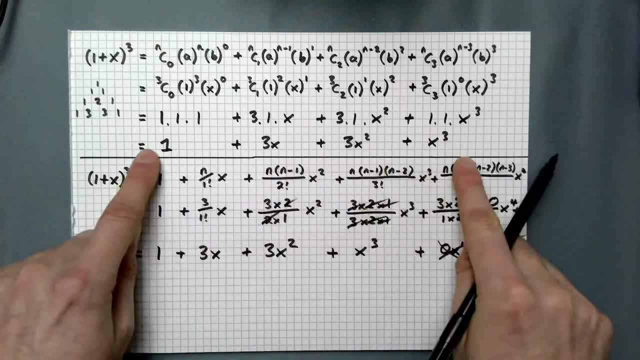 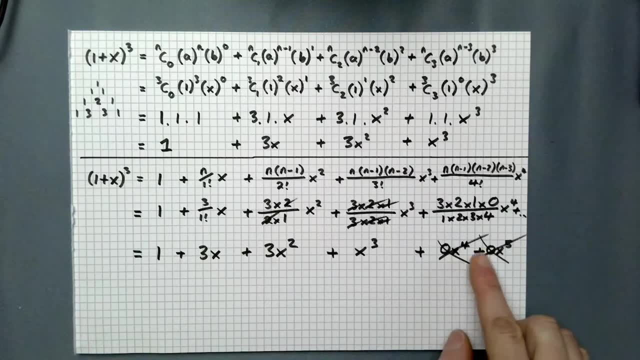 So I get the same answer overall if I use this new formula with a positive integer power. But the interesting thing that happens is that the term the expansion, if you will it kind of self-terminates, Because as soon as we get these 0 terms in our numerator, all remaining coefficients forever will become 0.. 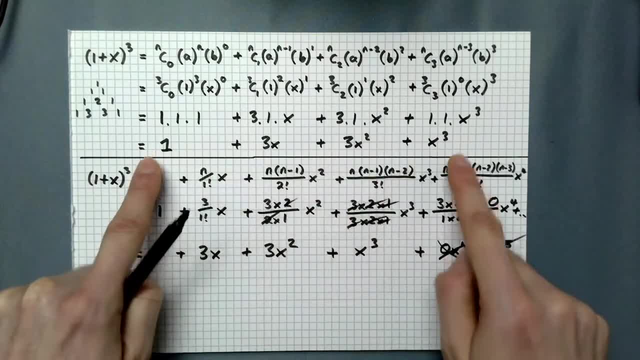 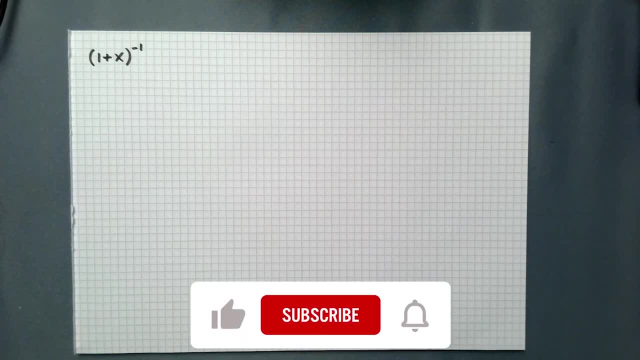 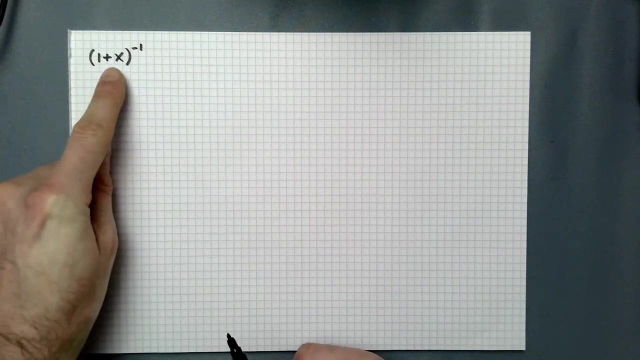 And we're just left with the same expansion as our original formula. So you might be wondering at this stage: why do we use the new formula then? Well, this new formula will work even if we have negative powers or fractional powers. Here I'm going to give you an example, using x plus 1 to the power of minus 1.. 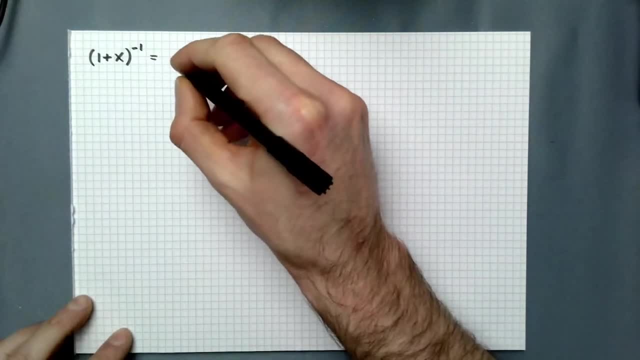 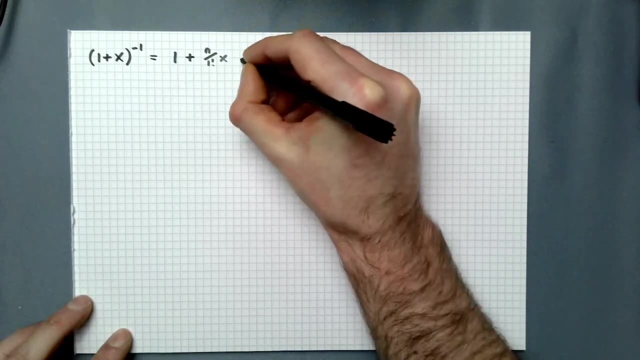 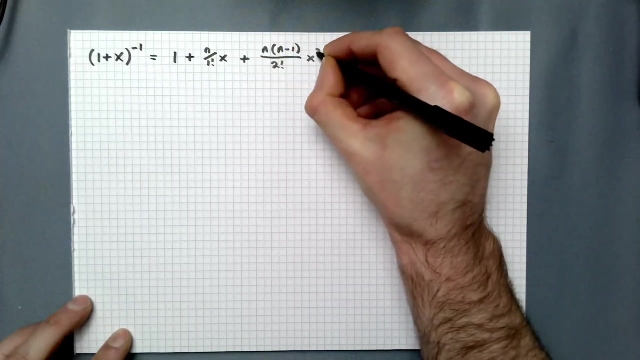 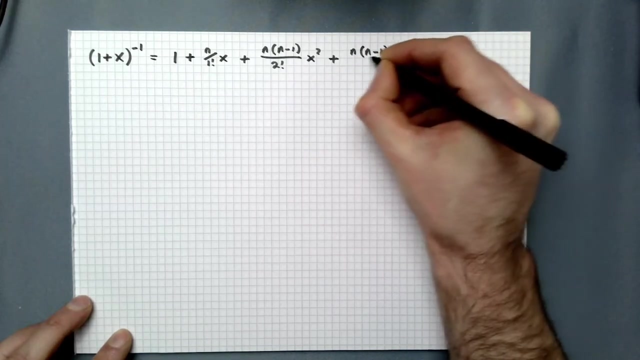 So if I were to plug this into my new expansion, my new formula: So 1 plus n over 1 factorial times x plus n times n minus 1 over 2 factorial times x squared Plus n times n minus 1. times n minus 2 over 3 factorial times x cubed. 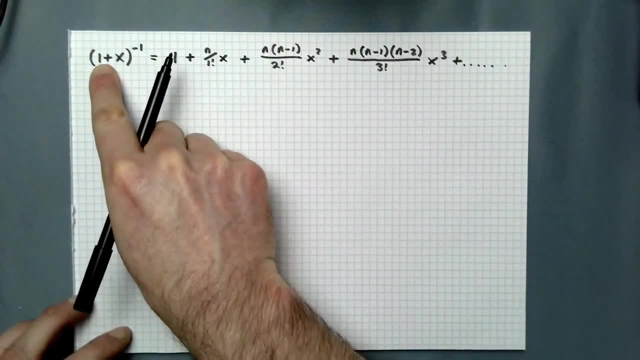 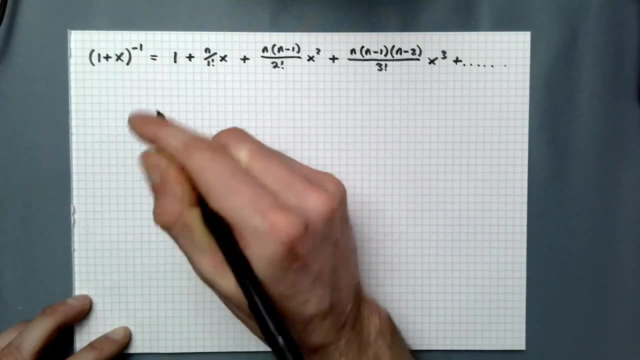 Carrying on and on and on. So I can see that I have a leading term of 1 in here, So I can use this formula, And I have an n value of negative 1.. So I have 1 plus negative 1 over 1 times x. 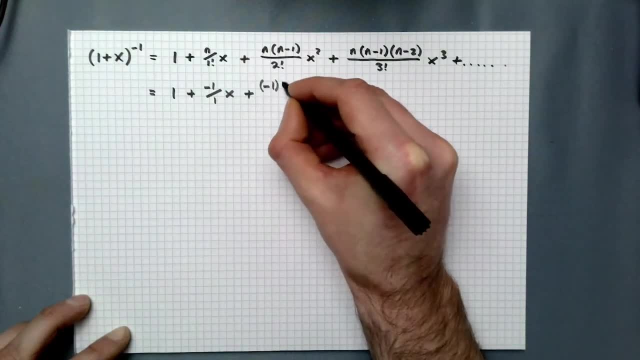 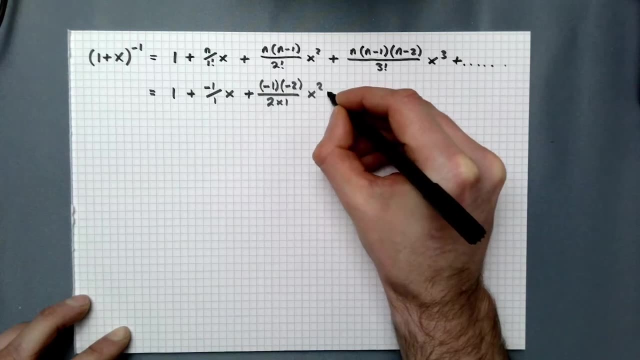 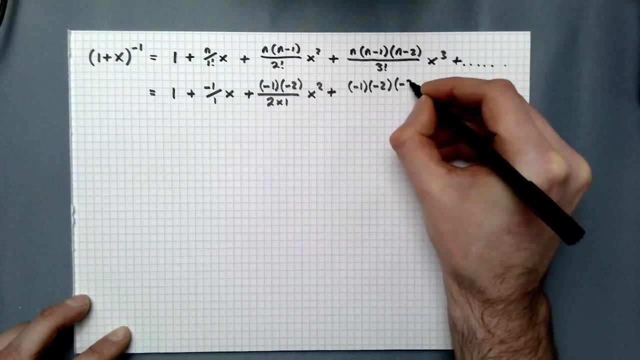 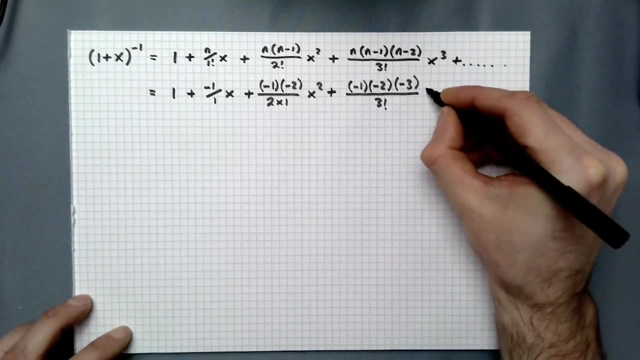 Plus negative 1 times negative, 2 over 2 factorial, which is 2 times 1 times x squared. Plus negative 1 times negative, 2 times negative, 3 over 3 factorial, 3 times 2 times 1 times x cubed. 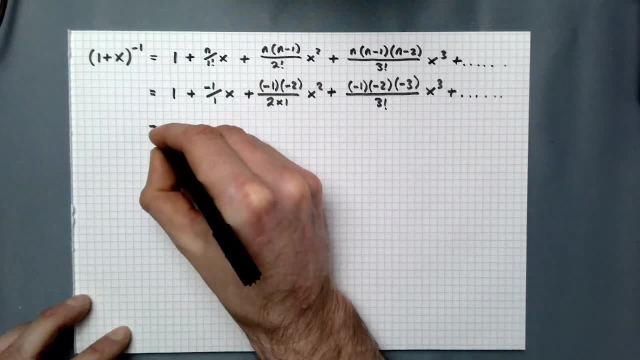 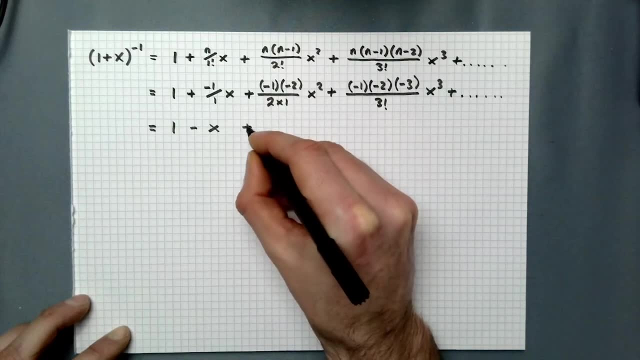 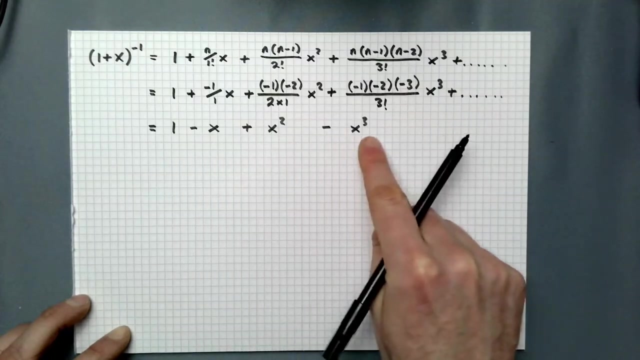 And this process will carry on and on. So I get 1 minus x, plus x squared, minus x cubed, And I think we're starting to spot a pattern here. So if I were to write out an extra term or two, 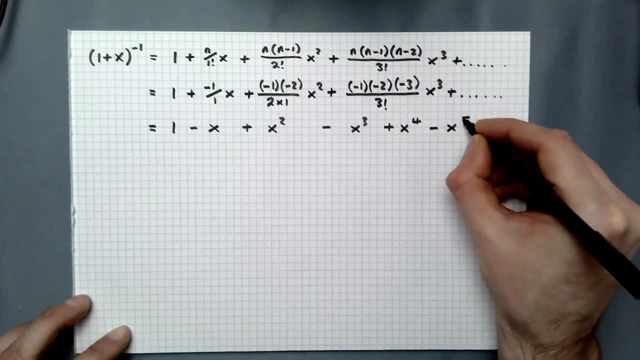 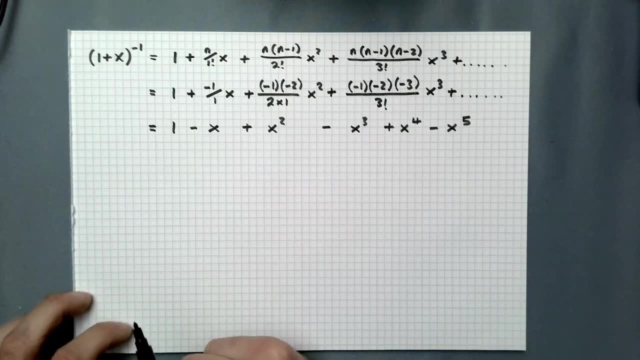 So plus x to the 4, minus x to the 5.. So these don't look particularly similar to each other, But something interesting happens And I can actually prove that these two terms are equivalent. So if I were to say 1 plus x to the minus 1.. 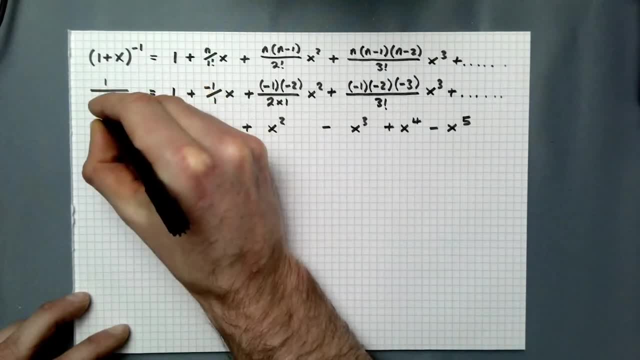 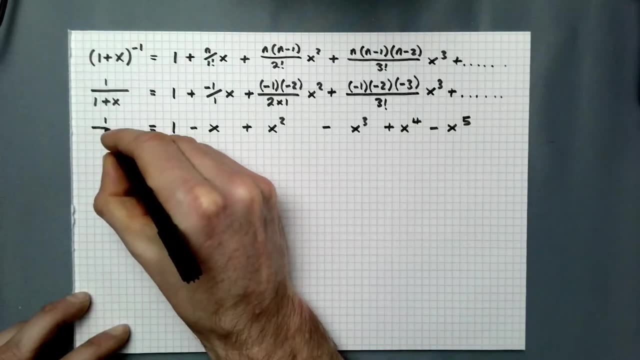 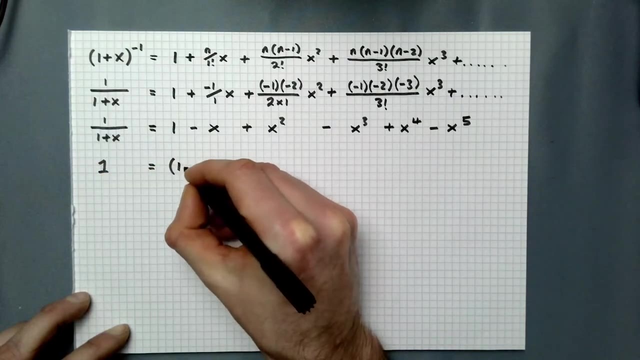 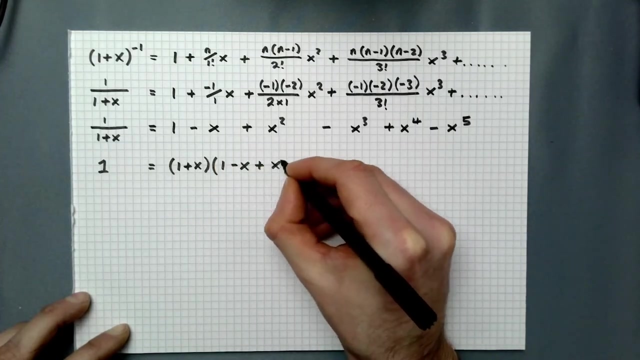 I can rewrite this as 1 over 1 plus x. So if I multiply both sides of this equation through by 1 plus x, I get 1 equals 1 plus x times by 1 minus x, Plus x squared minus x cubed. 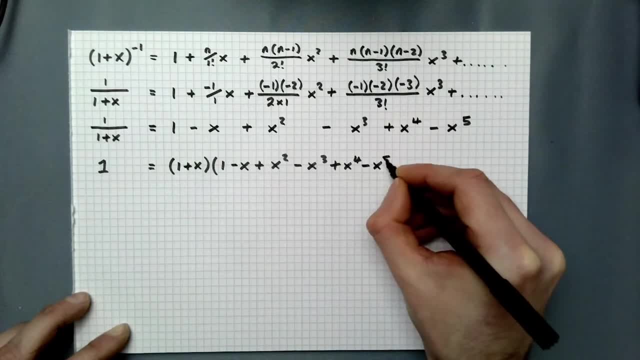 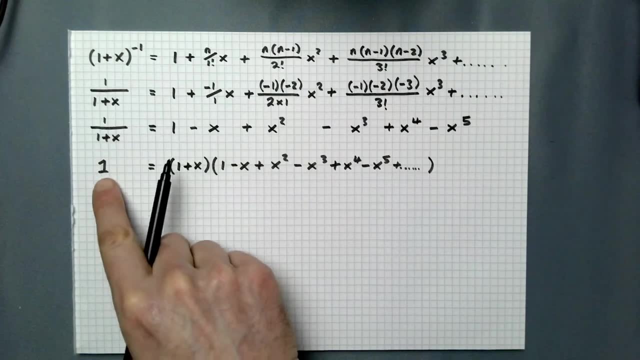 Plus x to the 4, minus x to the 5. Carrying on and on and on. Okay, so surely, if this equation holds, Then this would show that this expansion is correct And this formula is working for us. But I must confess, it really doesn't look like it's going to work for us. 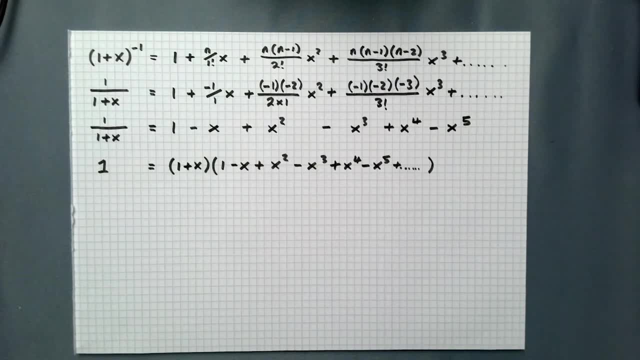 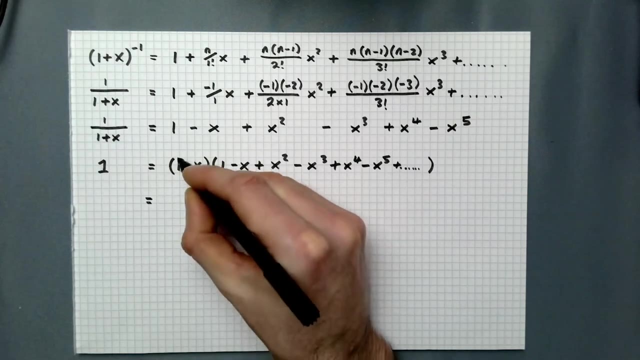 But you know, sometimes math might make you feel like you've backed into a bit of a corner. Try it anyway. Try expanding brackets, Try plugging in terms, Try spotting patterns. Let's see what happens if we expand these brackets. So 1 times 1 is 1.. 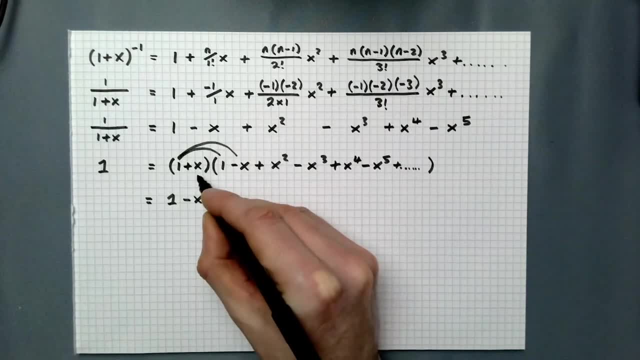 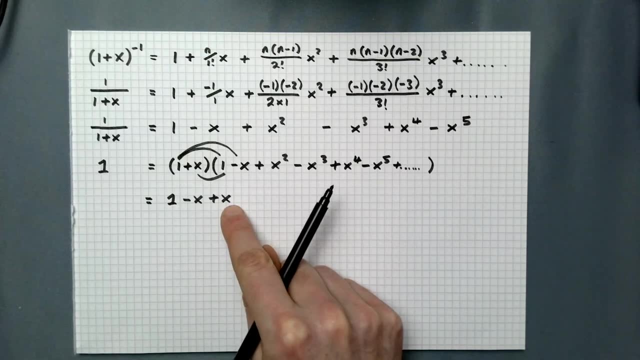 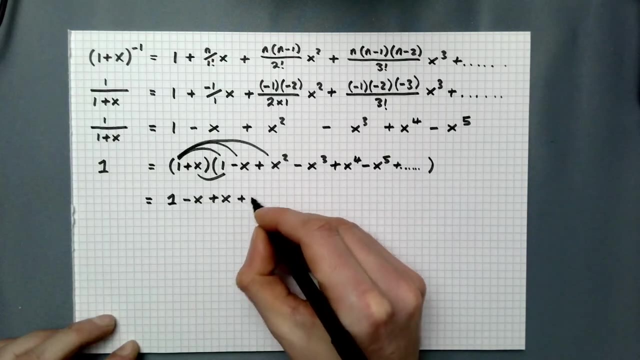 1 times by minus x. Positive x times by 1.. Oh Well, it looks like they're going to cancel out. Okay Well, let's keep going. So 1 times by x squared Is x squared Plus x times by minus x. 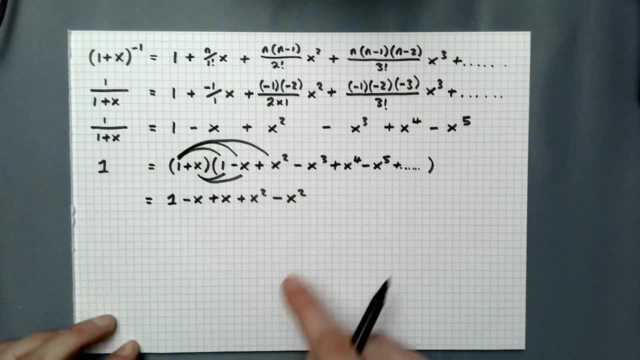 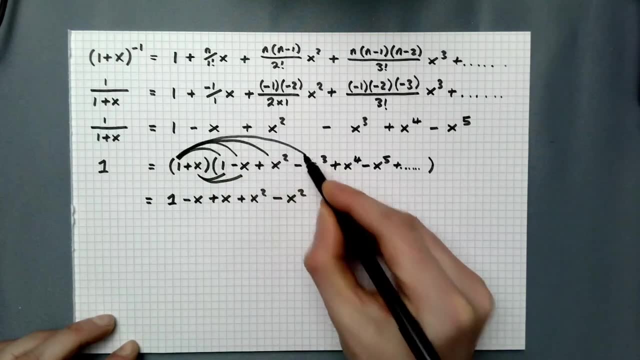 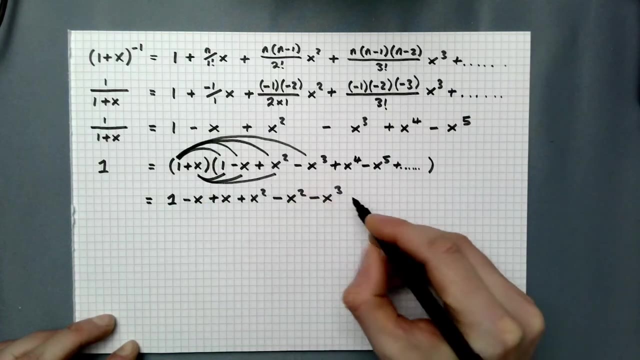 Is minus x squared. Well, it looks like they're going to cancel out as well. Great Carrying on 1 times by x cubed. Sorry, 1 times by minus x cubed Is minus x cubed And x times by x squared. 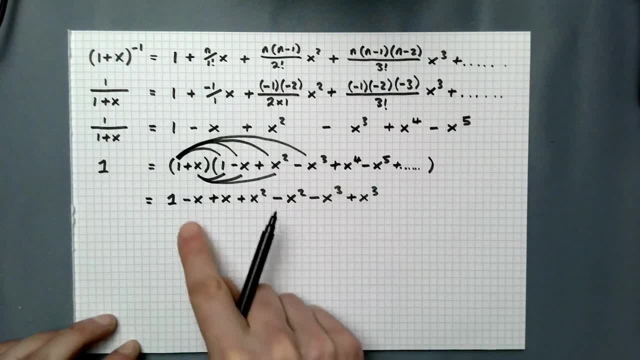 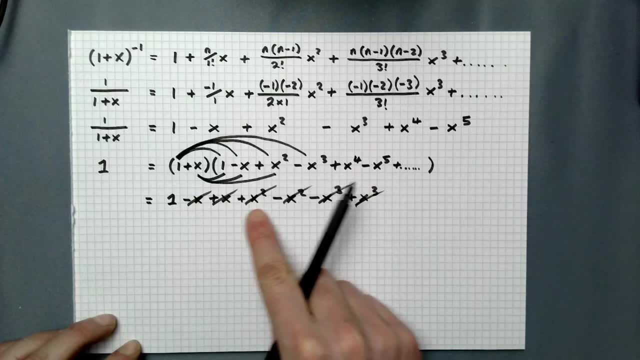 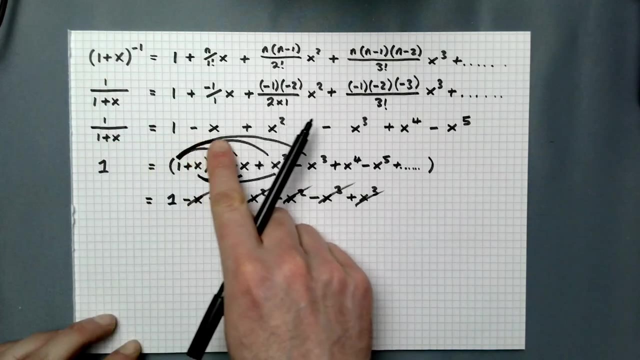 Is positive, x cubed, And this pattern will carry on. These two terms are going to cancel. These two terms are going to cancel. These two terms are going to cancel. This pattern's going to carry on forever. So what this shows us is that this expansion for 1 plus x to the minus 1 is perfectly valid. 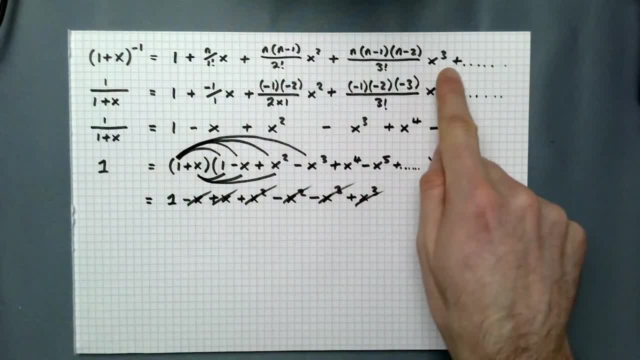 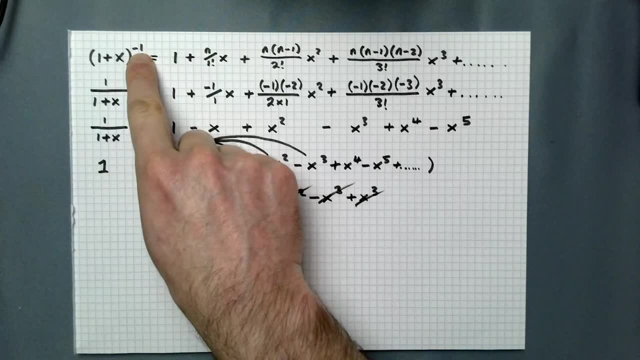 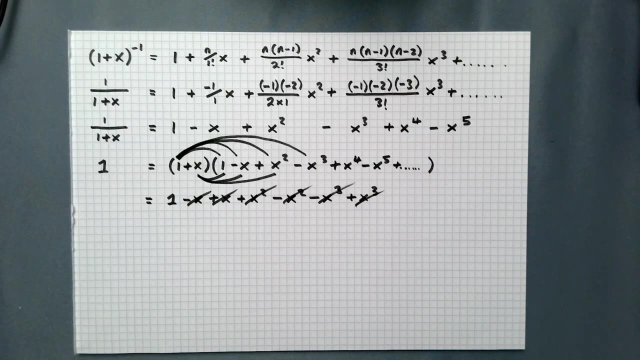 So we have shown here That this new formula that we've developed does produce valid expansions even when we have non-positive integer powers. So I'm going to wrap that up for this video, But in the next few videos I'm going to kind of expand on this a little bit. 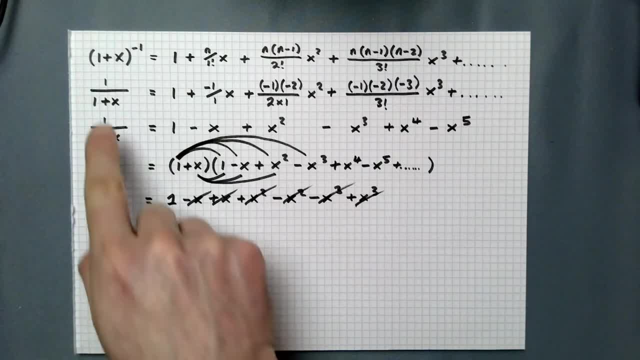 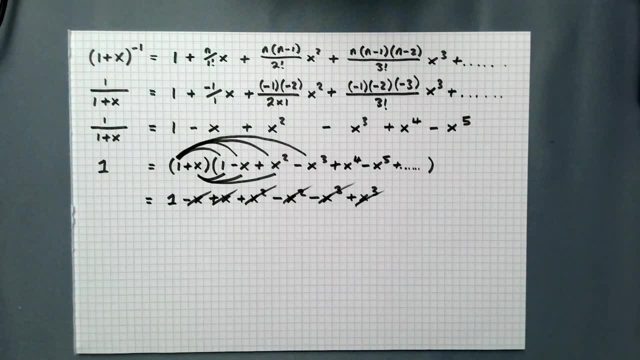 I'm going to do loads and loads of examples, Particularly what happens when we have a leading term that isn't 1 within our brackets, And also when these expansions can be used to make approximations. So I will see you in the next video. 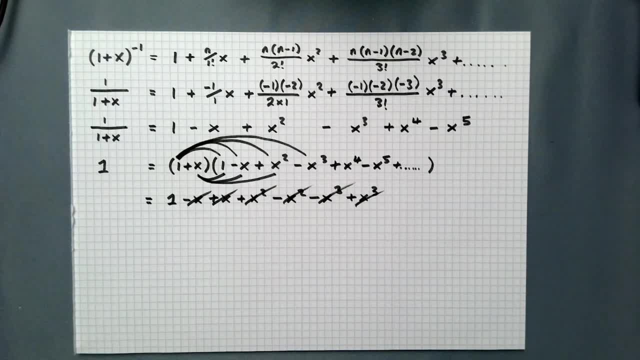 If you've got any questions or comments, please do leave them down below, And I will see you soon.